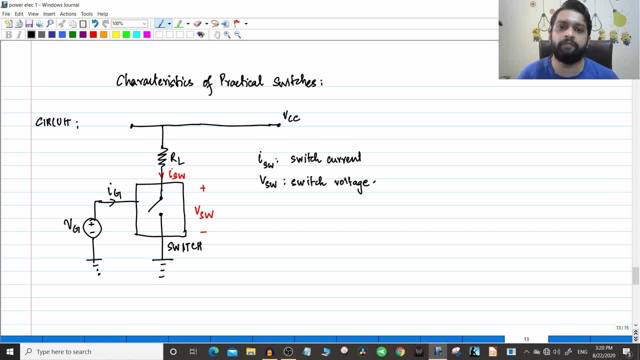 user as well, as it should have good characteristics, resembling an ideal transformer, right. So today we will start with the practical switches. So I want you to go through this circuit very closely. So you are having a voltage source, Vcc, and the load RL is connected. 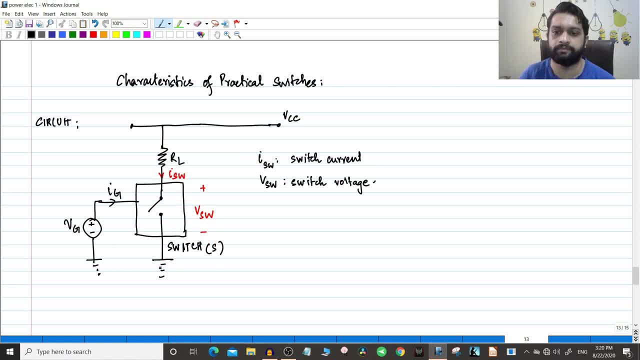 through a switch. you can call that switch S to the ground, okay, And then to turn on and turn off the switch, you are having the Vg and Ig, So we will write down that. So Isw is a switch S. 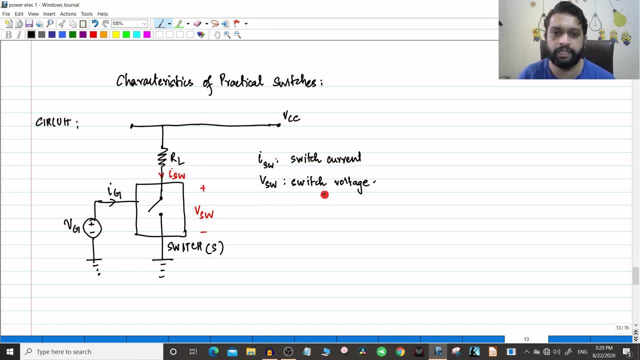 current Vsw is the switch voltage. the voltage across the switch is called switch voltage. You do not need the voltage across the resistance for this particular explanation, So we are not going to consider that. But, however, we will be considering the current which is flowing. 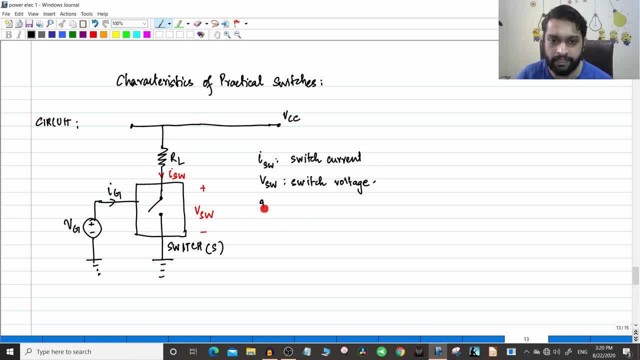 through the switch here. Now, other than that, you can see that Vg is the gate voltage and Ig is the gate current. So you know what is the condition. In this particular condition you can see that the switch has proper biasing and all. So the Vg, when Vg is on, and Ig. 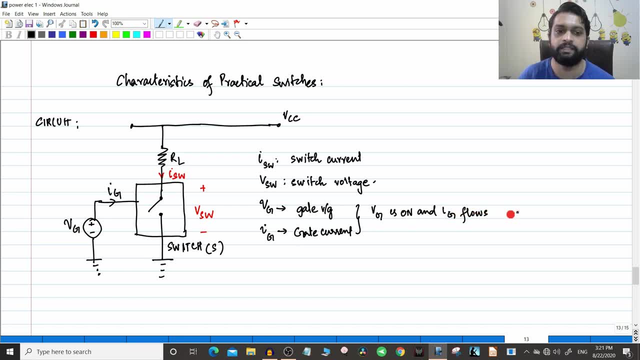 flows. Vg is on and Ig flows. the switch S1 is on And the when the Vg is off, Vg is off. Vg is off off and Ig stops. Ig stops flowing. switch S1 is- we can call that S1, switch S1 is off. 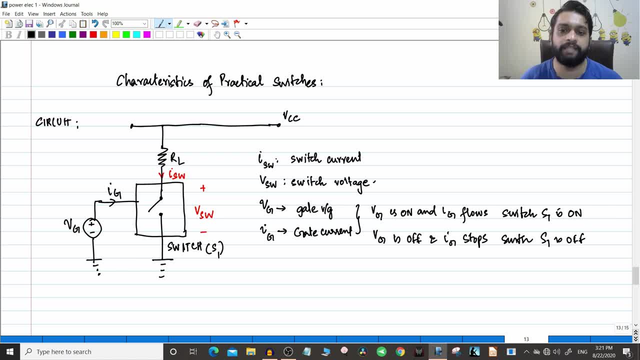 So we will now write down what will be the voltages and currents etc when switch S1 is on. So we will write down that here. So when S1 is on, let us see what will be the voltages. So when S1 is on, you can see that the switch will be closed legs. So we will 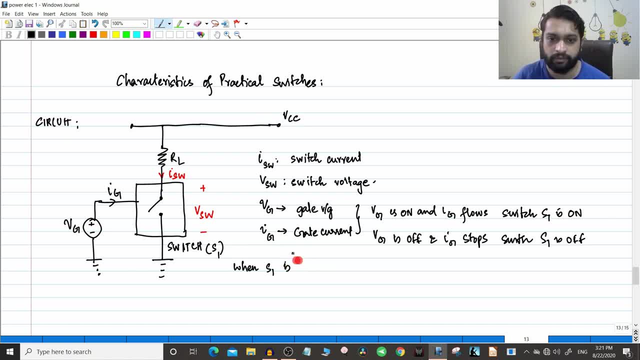 write first when S1 is off, so that I can prevent one rubbing here. So when S1 is off, so this switch is open. switch is off condition, so it is open. So if you see, if you apply a little bit of KVL here, you will find out that Vsw will be equal to Vcc and Isw will. 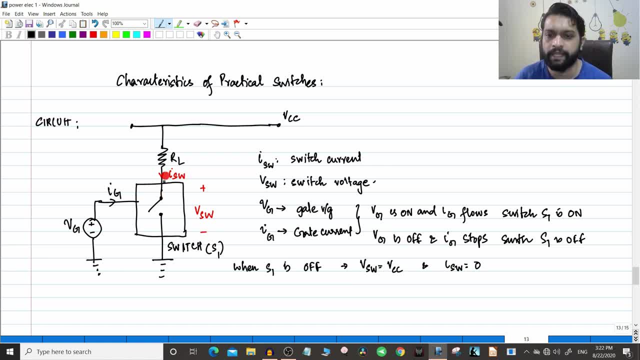 be equal to 0.. Naturally, when the switch is off, condition there will be no current flowing through. it is open circuit Now when S1 is on. So when will be the S1 be off? S1 will be off. you know that when Vg is off, When Vg. 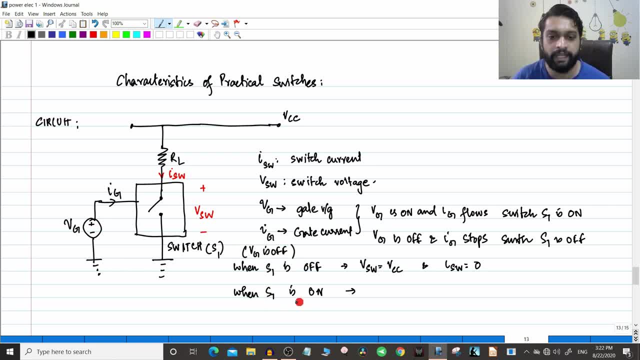 is off, or you can tell that when Vg is equal to 0.. And when will S1 be on? When Vg is on or when Vg is not equal to 0.. We will see that in a graph shortly. When S1 is on you. 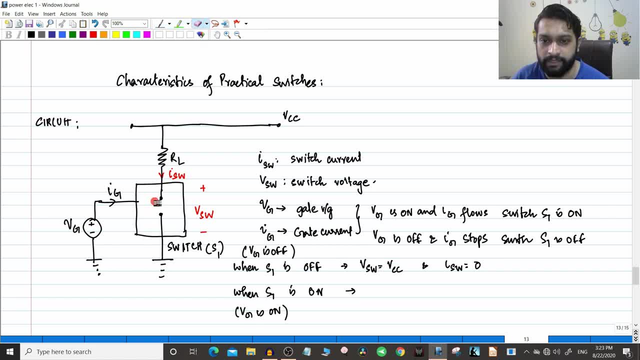 can clearly see. we can write, do something like this, We can rub this here. So this is not an open circuit. When S1 is on, it is a short circuit here, So the switch is closed. So you can clearly see from here, if you see, measure the voltage for an ideal switch Vsw. 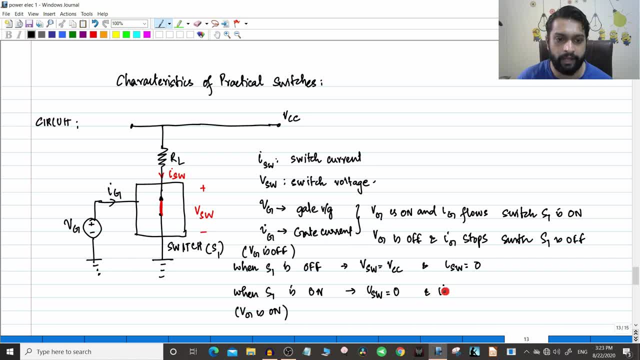 will be equal to 0.. And what will be the Isw value? Isw value will be equal to Vcc divided by RL. Now we will just draw this in form of a graph So that when we draw the graph for practical switches it will be much easier to understand. 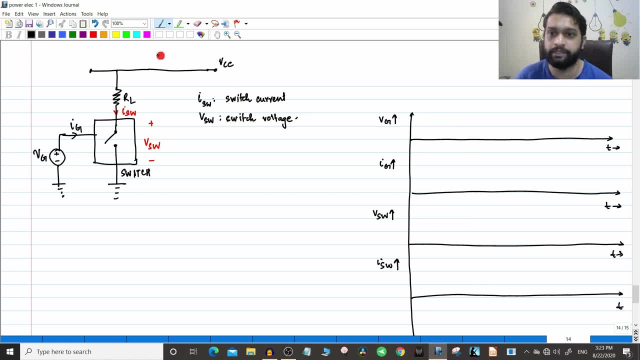 So I have already made some diagrams here. So what we are going to do is that we are going to turn off the circuit. We are going to turn off the circuit, We are going to turn on the Vg value. That means, for example, let us wait till this time here, So at time. 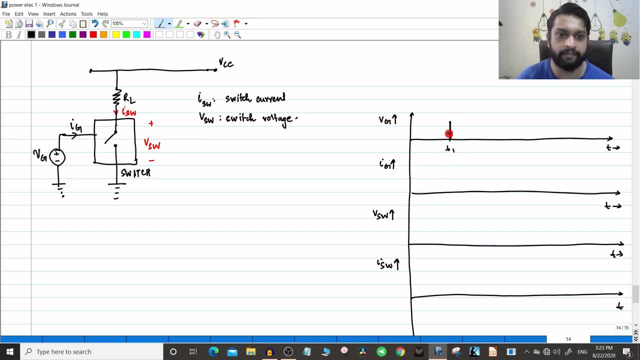 t1, we are giving a gate signal, We are giving a gate signal And let us assume that as long as, as long as the gate signal, gate signal is not equal to 0, the switch S1 is on, And when the gate signal is equal to 0, the switch S1 is off. So this is the condition that we 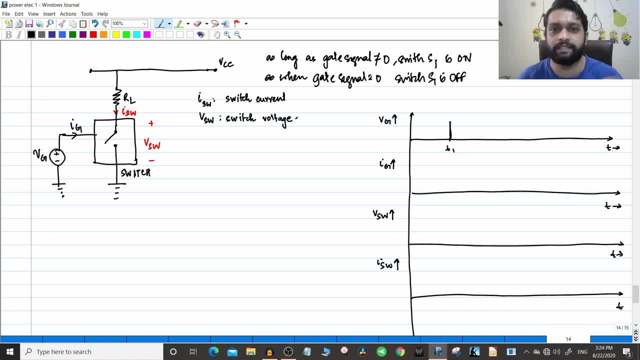 are going to use. I have already told you in the ideal switches that we usually use pulsed triggering, But for this explanation we are not going to use pulsed triggering. We will assume that as long as the gate signal is there, S1 is on, And once you remove the 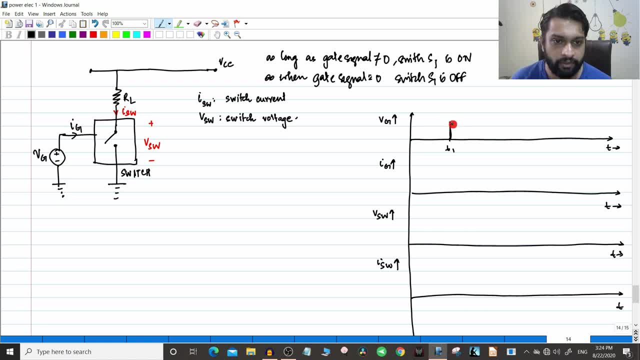 gate signal. the switch is going to be off. So let us take it till this here. So we are applying Vg till at this point here. So you can clearly see that Vg is not equal to 0 at this point. Vg is equal to 0 at this point, And beyond this also, Vg is equal to 0.. So 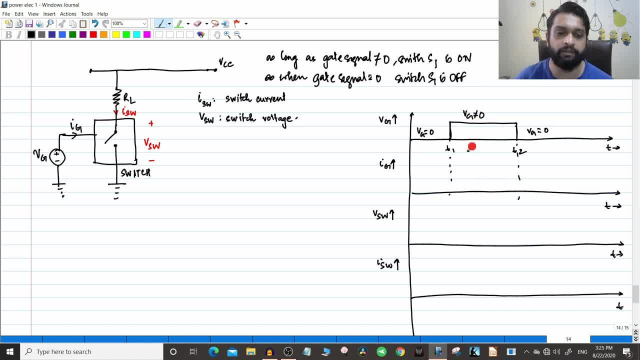 this is t1 and let this be t2.. So if Vg is not equal to 0, naturally some Ig also will be flowing. So this is the value of Ig. So look at this very carefully. So at time, t1,. 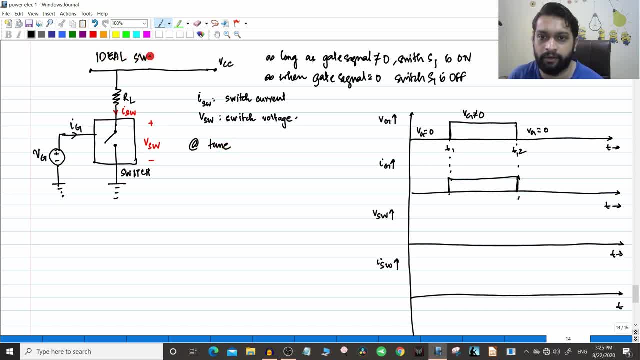 so now we are talking about ideal switches. So for the time being we are talking about ideal switches And once we draw the graph for the ideal switches it will be very easy to understand the practical switch. So at time t1, Vg is applied and Ig flows, That means what is the meaning? at time t1, the 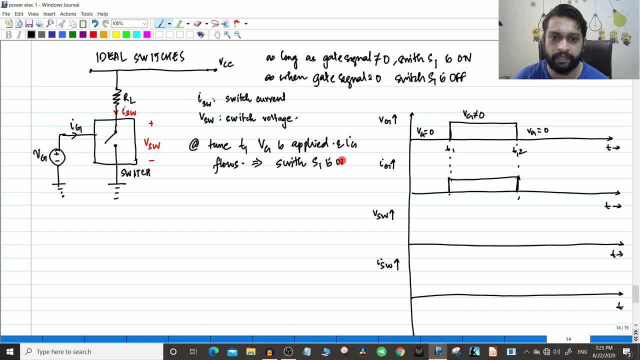 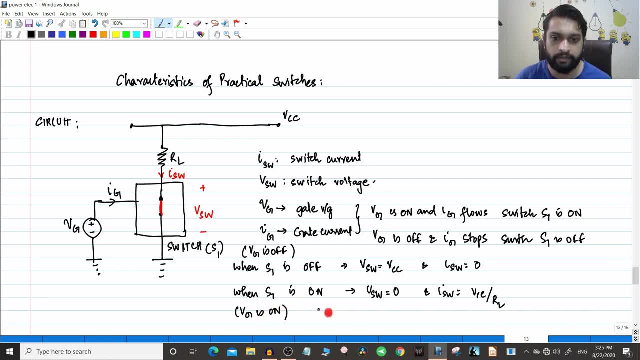 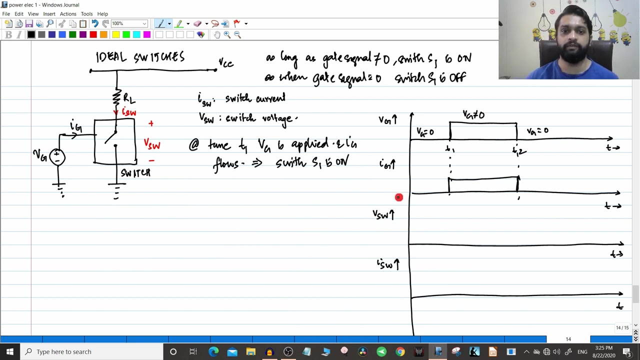 switch S1 is on. Switch S1 is on. See, already we have seen whenever the Vg is on. So we have seen that whenever Vg is on, the switch S1 will be on. When Vg is off, the switch S1 will be off. So that we already know here Switch S1 is on. So now we will. 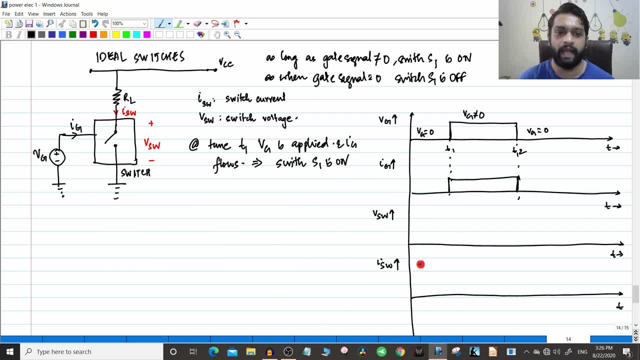 draw, for different time intervals, the graph of Vsw and Isw. So we will just make the graph here like this: In power electronics. see, you have to remember that drawing graphs is very important And you have to try to make them as neat as possible, Because in power electronics graphs are very 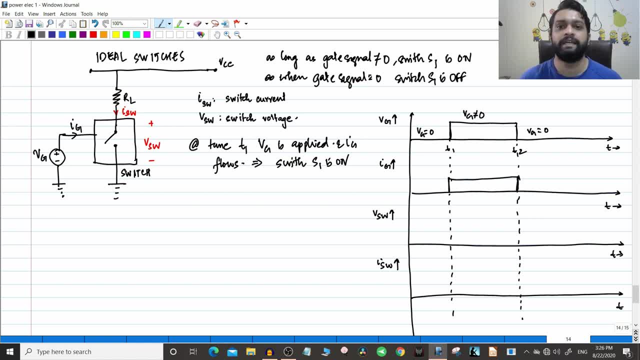 very important to analyze, And if you do not draw your graphs neatly, you will lose interest in the subject. So make sure you have a paper with you And you possibly, if you can use a scale or something like that, you can use that, or if you are good in freehand drawing. 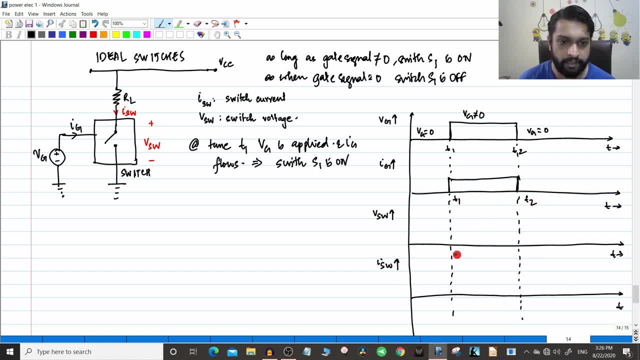 you can do that. So this is t1,, this is t2.. Here also t1,, here also t2, t1, t2.. So let us take the first time interval: 0, less than t, less than t1.. This time interval from 0 to t1.. So from 0 to t1,. 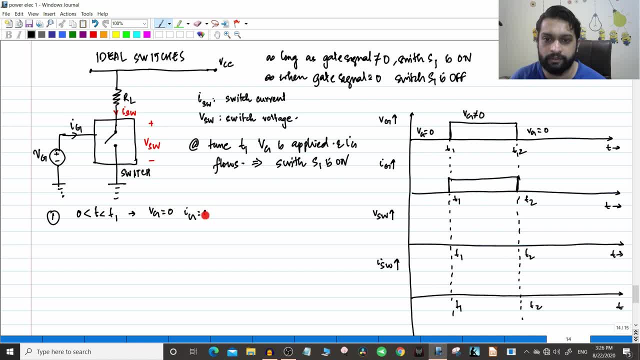 you can see, the Vg value is equal to 0, Ig value is equal to 0. So when Vg is equal to 0 and Ig value is equal to 0, the switch S1 is off, Whenever Vg is equal to 0 and Ig is. 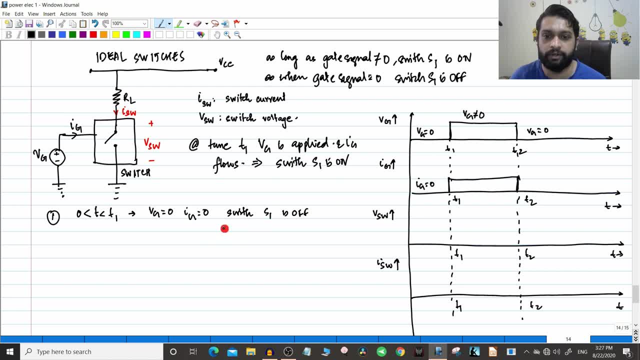 equal to 0,, switch S1 is equal to off, And when switch S1 is equal to off, you know what is the condition will be equal to Vcc, Vsw will be equal to Vcc and Isw will be equal to 0. So I will draw the. 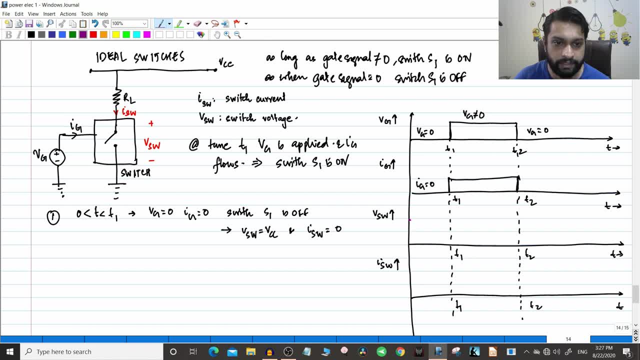 graphs for voltage here. So Vsw is equal to Vcc. So let this be: Vcc 0 to T1, Vsw is equal to Vcc and Isw is equal to 0.. Isw is equal to 0 from 0 to T1.. So this is for an ideal switch, Remember. 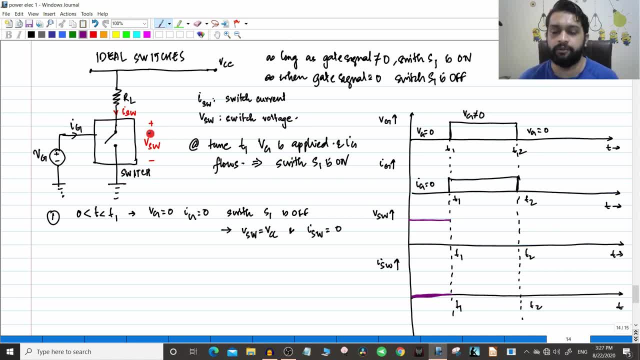 that this is for an ideal switch, what we are talking about. So we are not having any leakage current and we are not having any forward voltage drops. All these conditions are not present here, So that is why Isw is equal to 0. Although switch is 0, there is no leakage current. That. 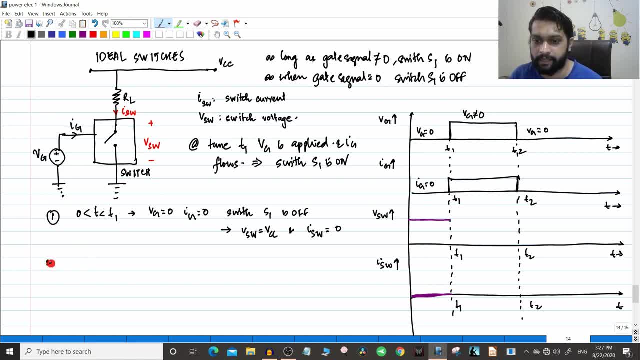 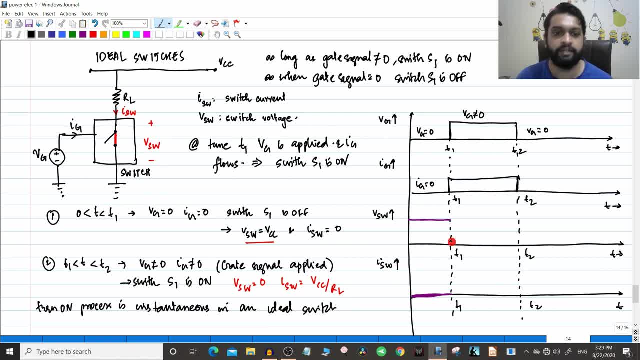 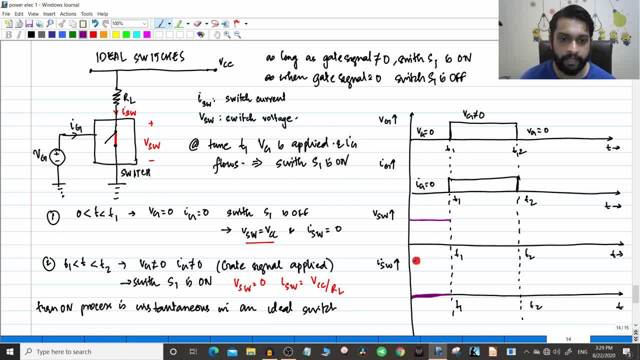 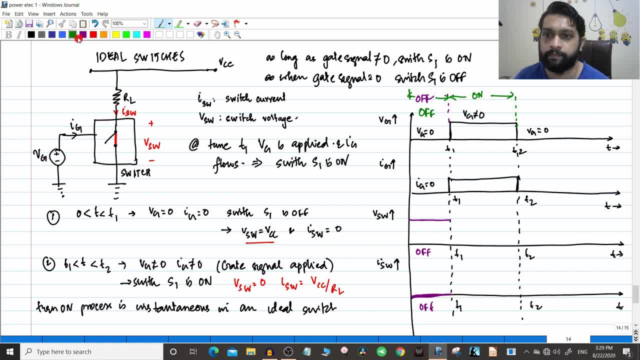 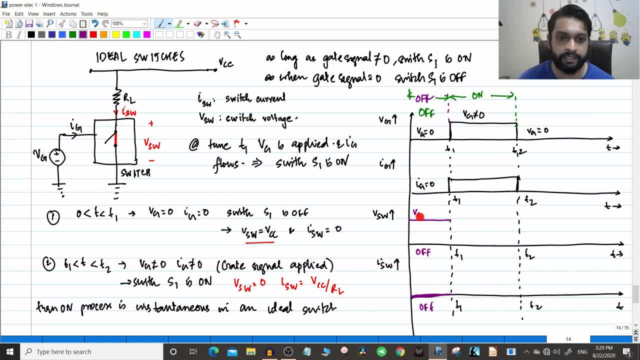 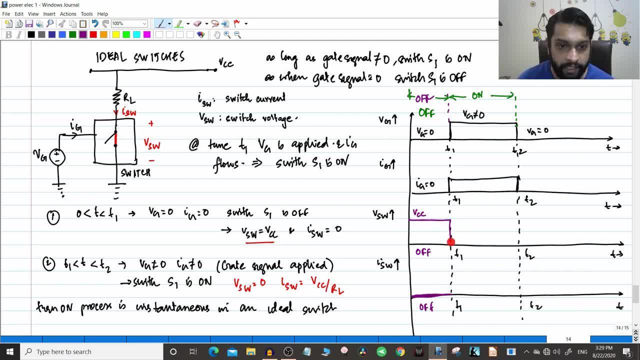 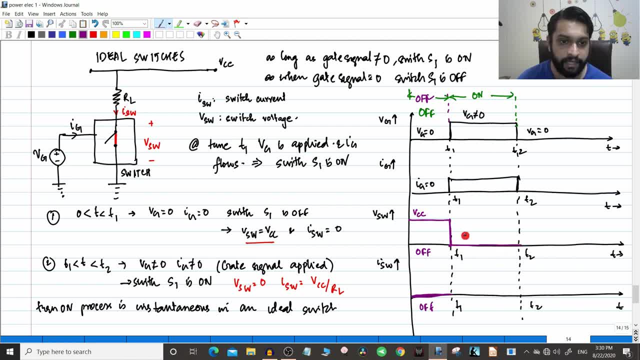 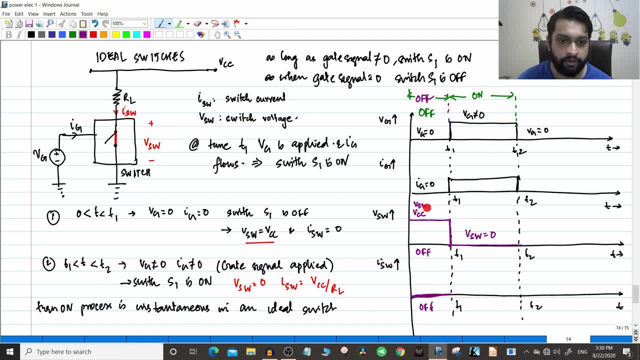 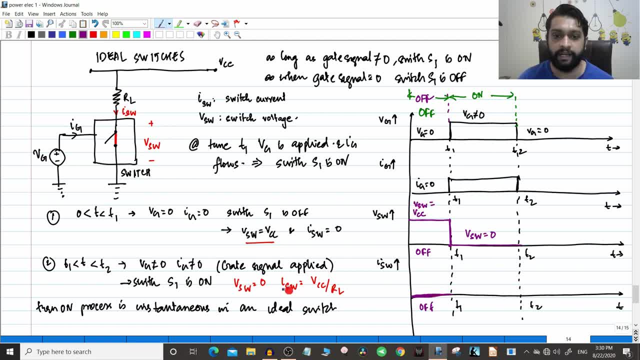 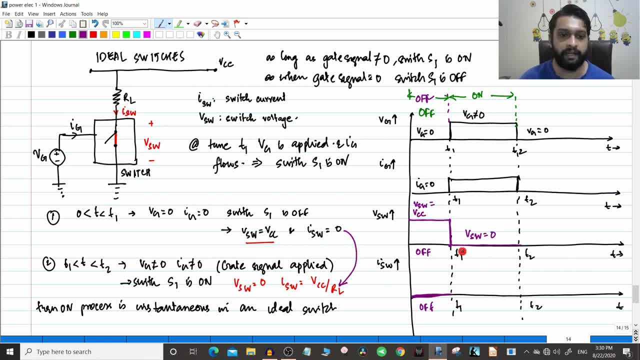 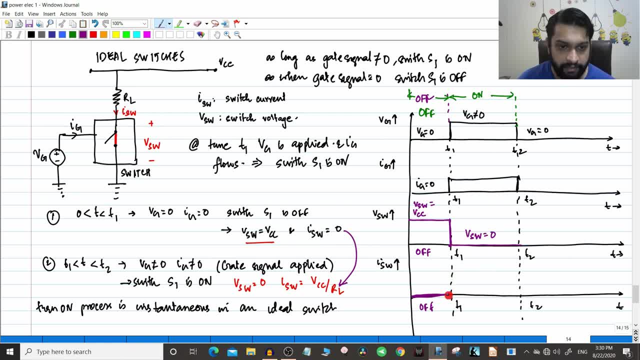 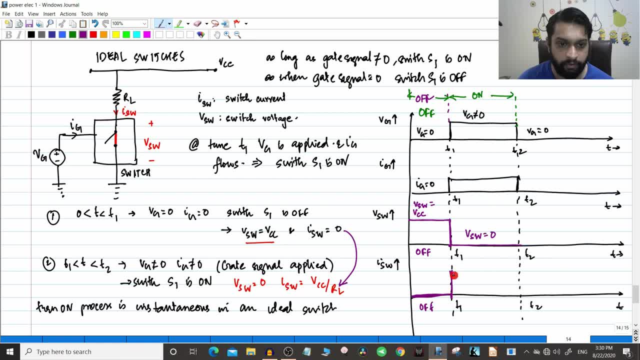 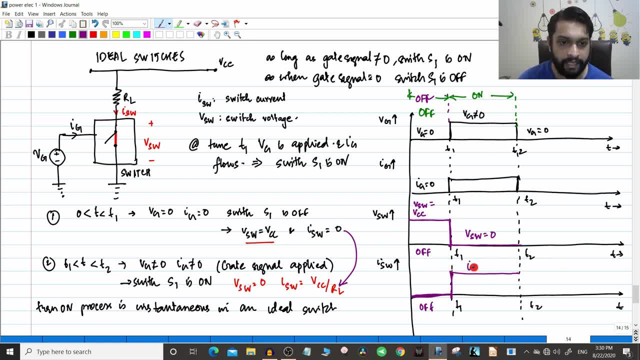 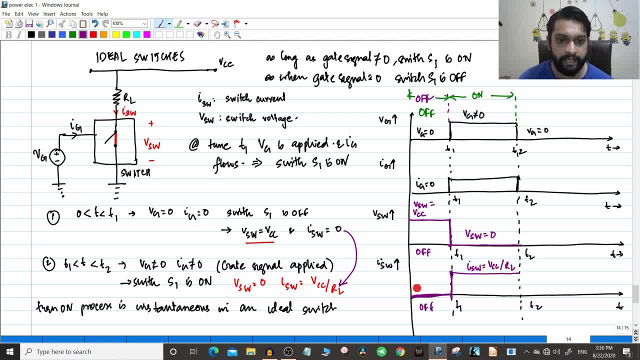 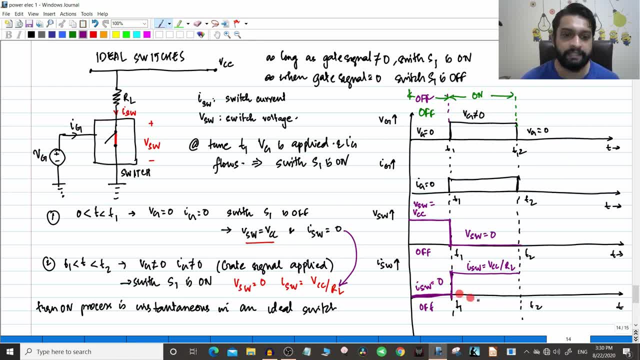 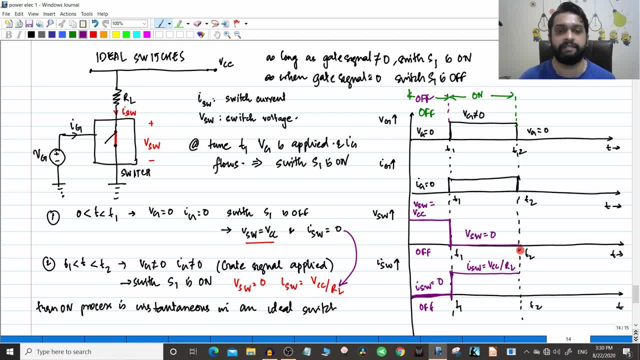 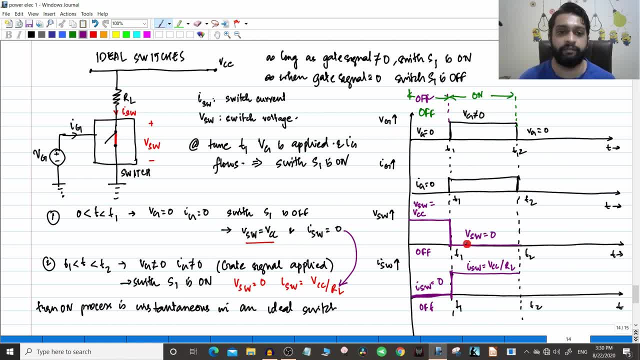 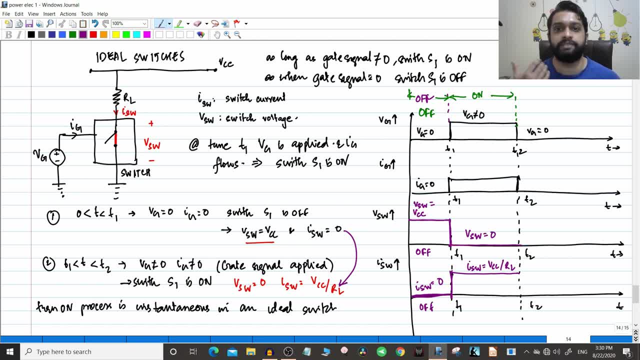 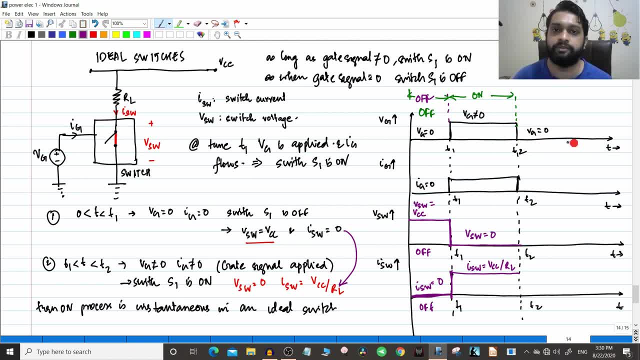 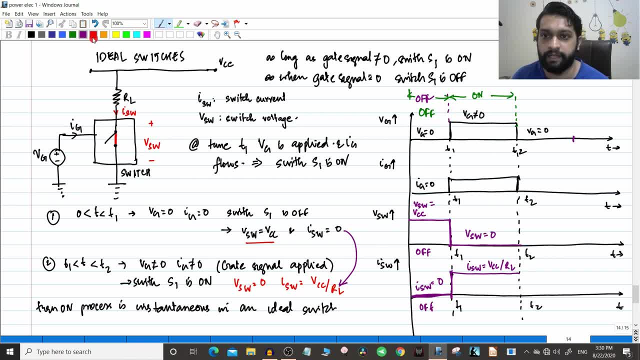 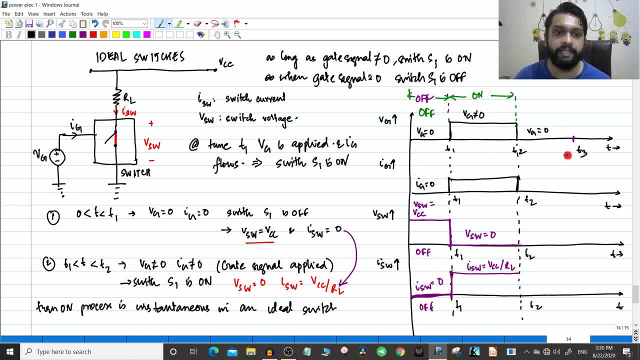 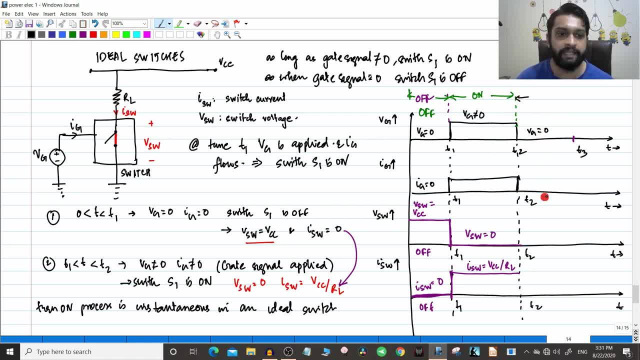 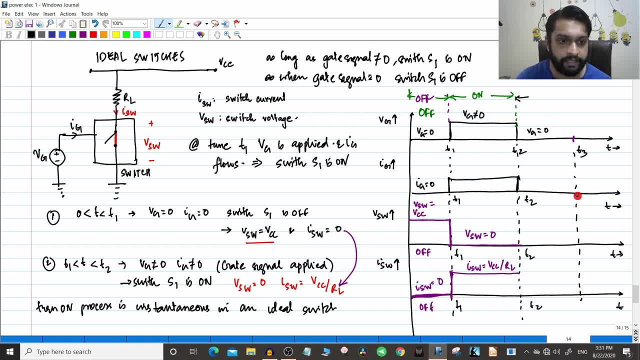 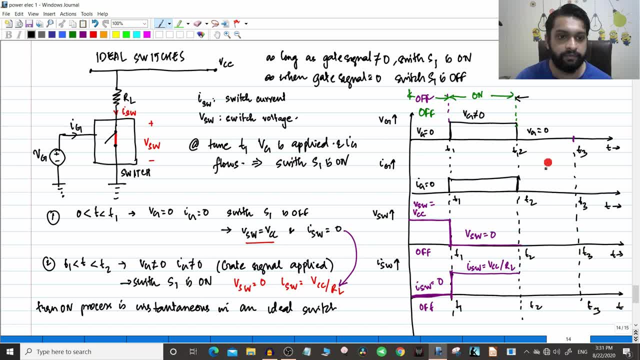 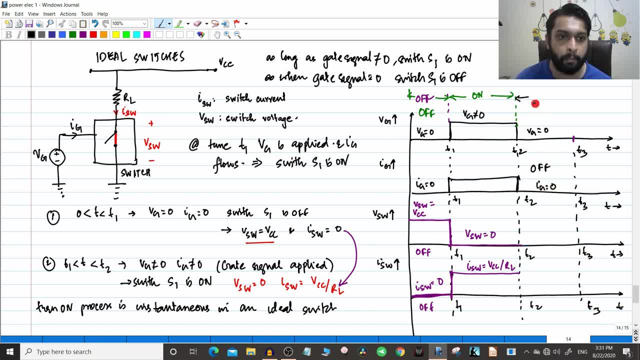 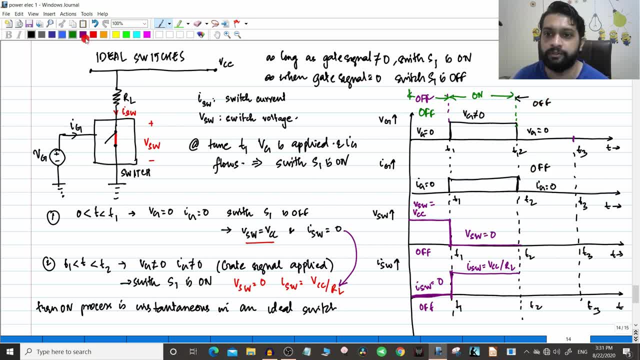 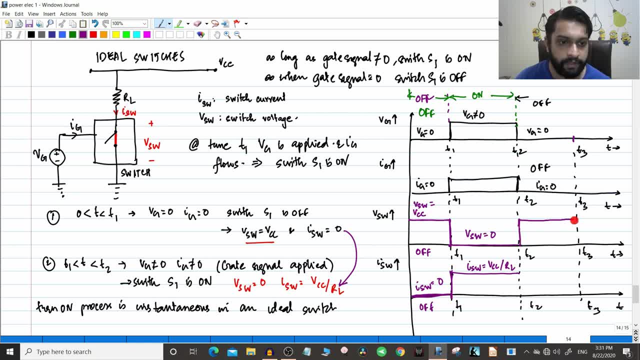 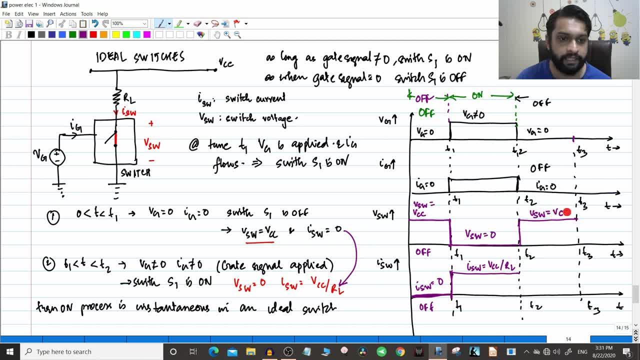 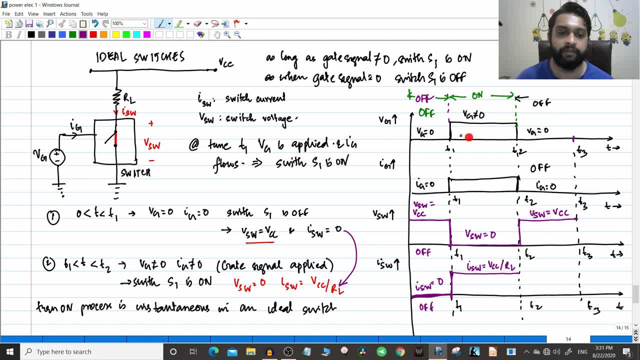 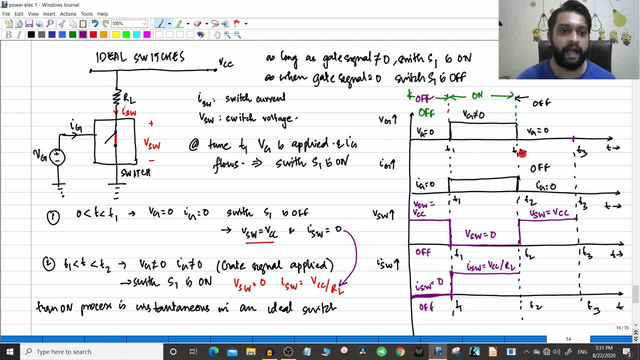 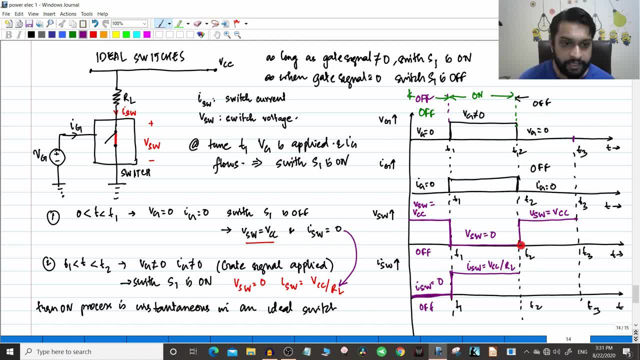 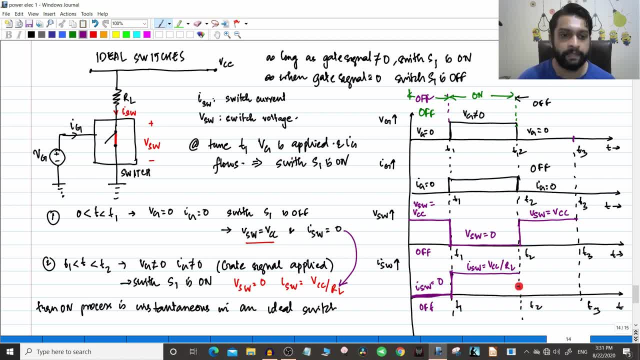 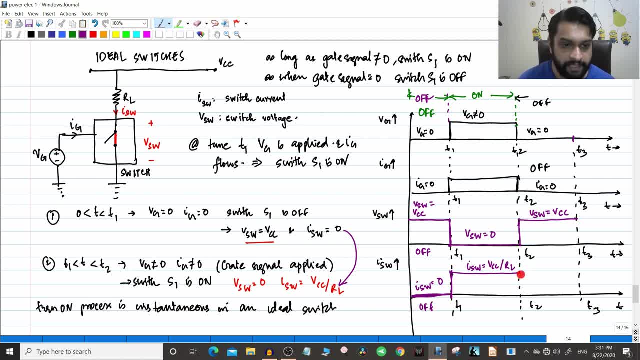 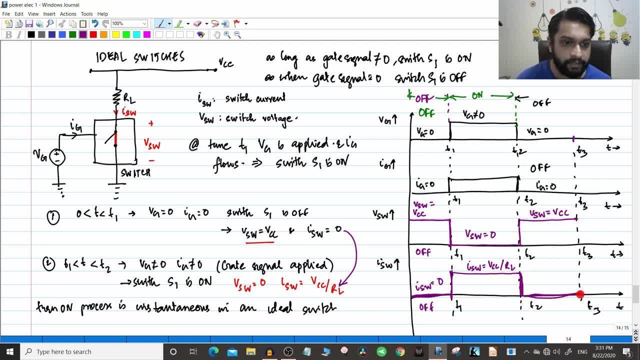 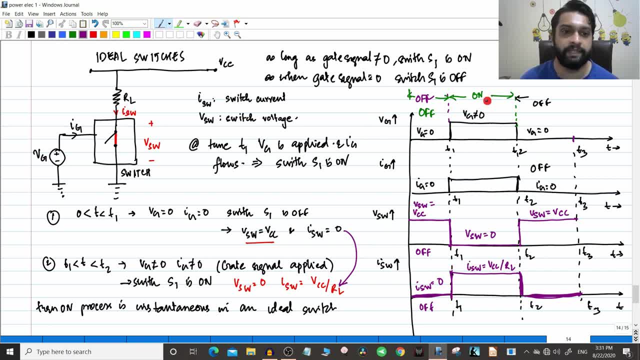 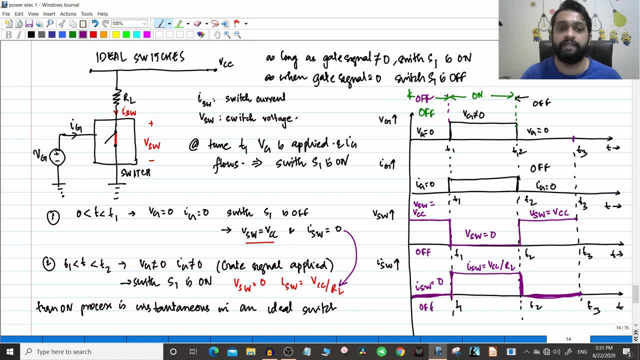 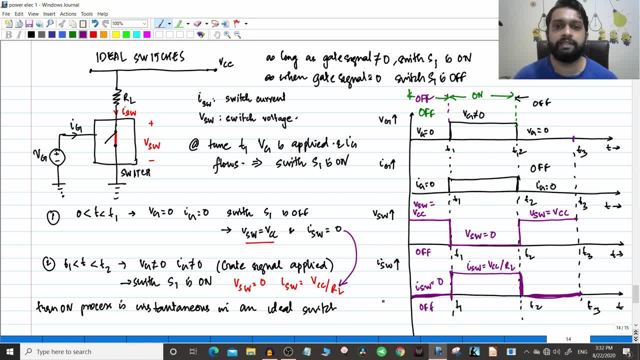 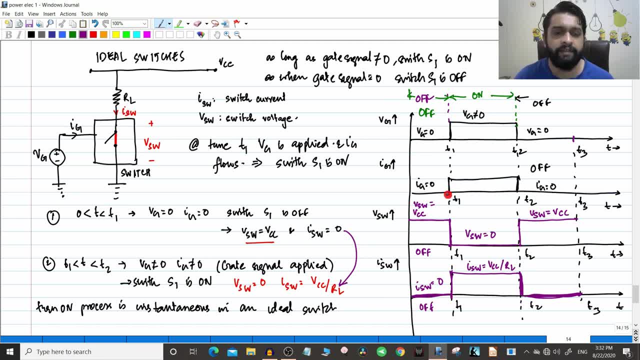 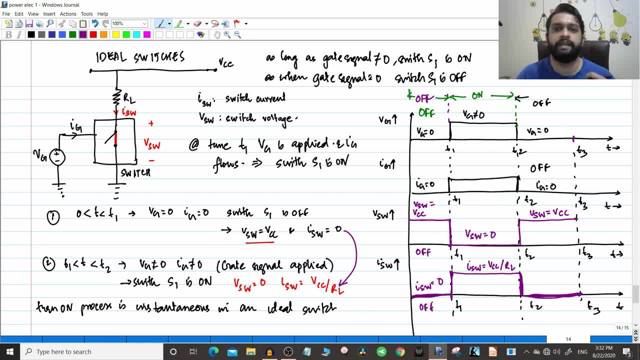 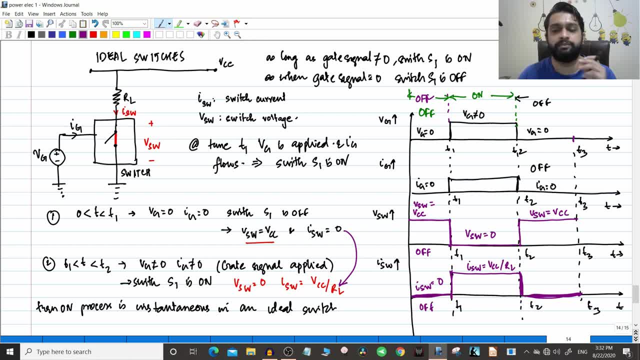 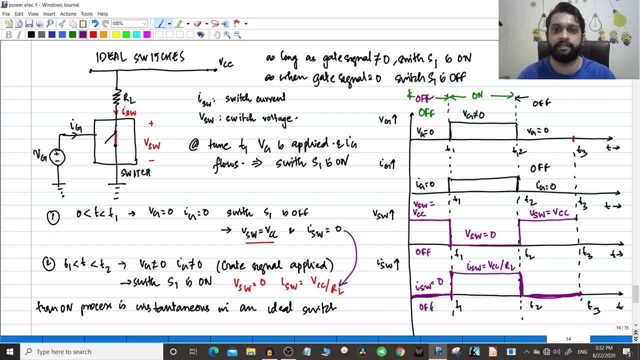 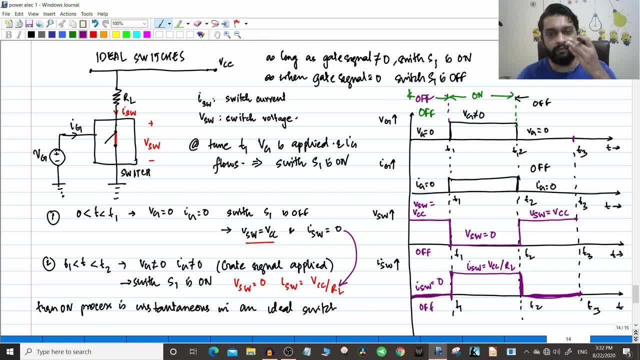 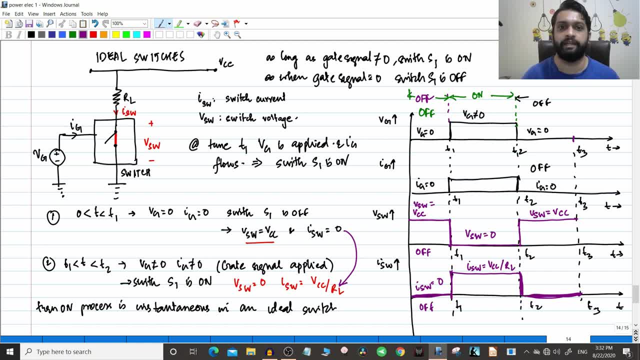 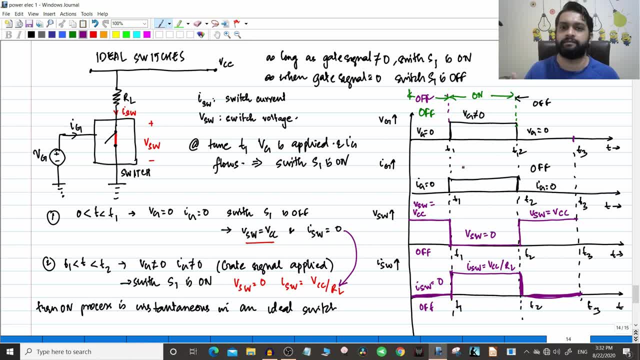 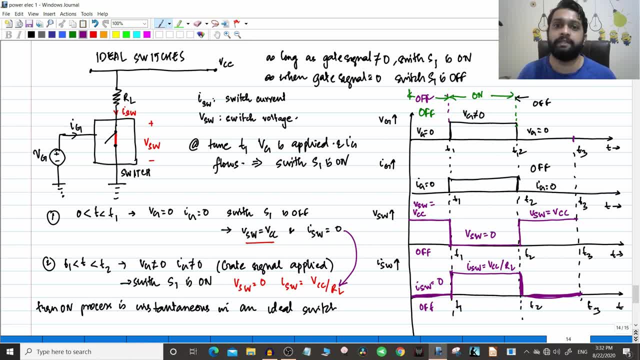 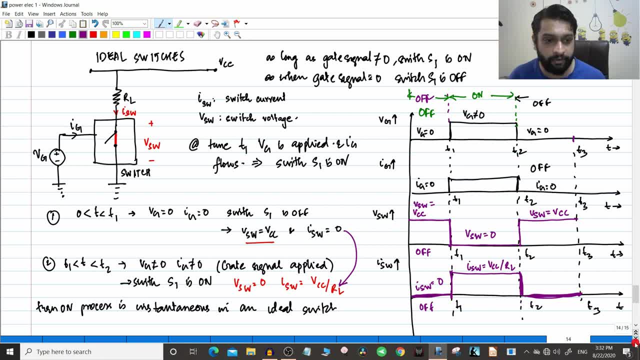 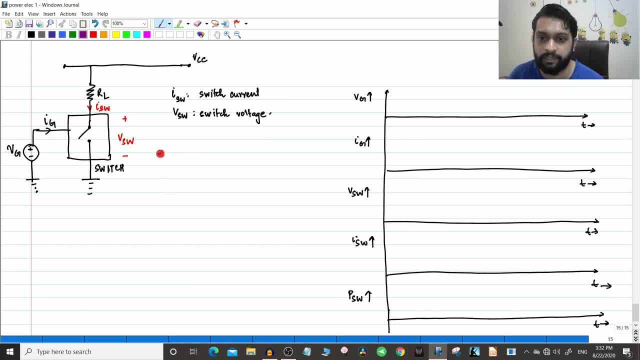 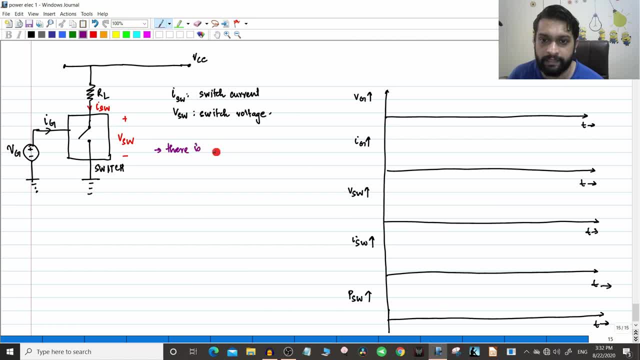 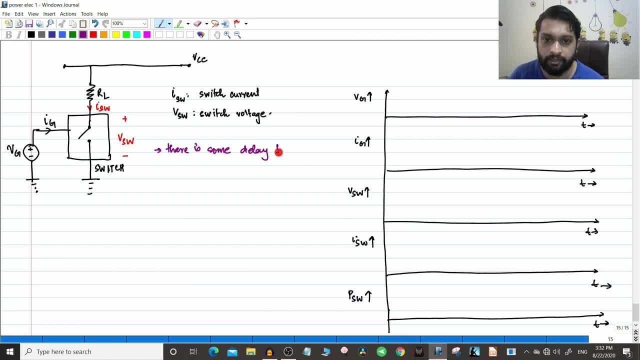 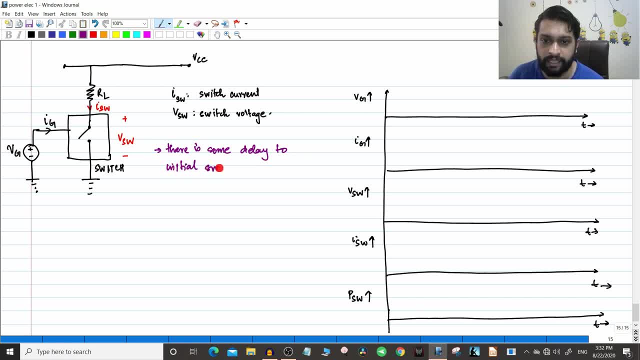 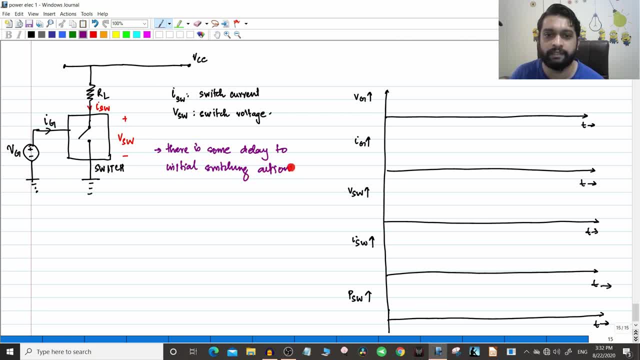 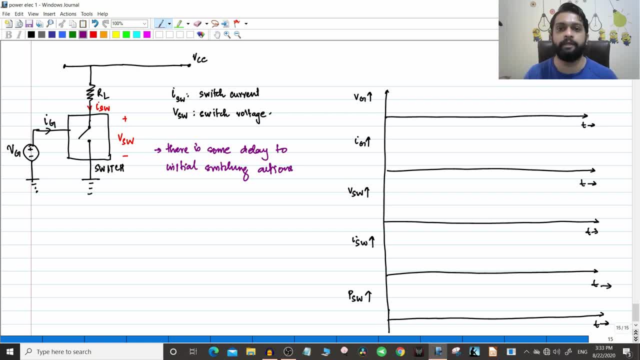 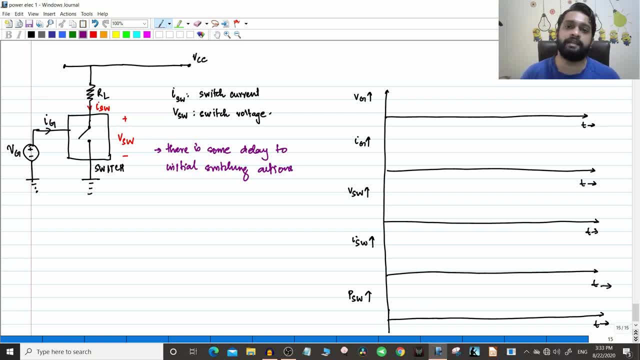 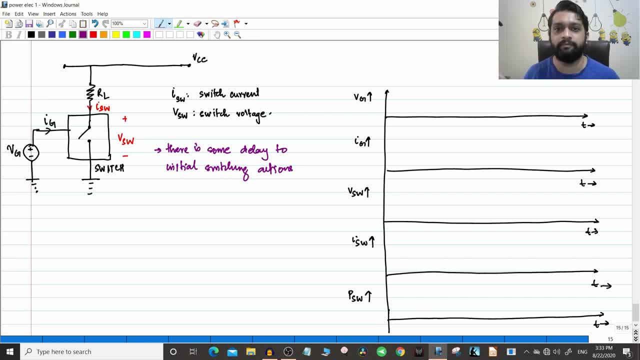 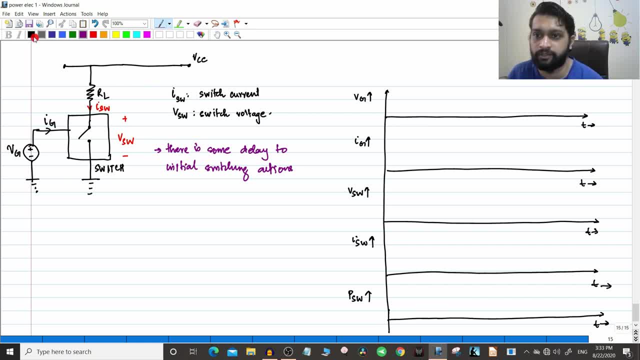 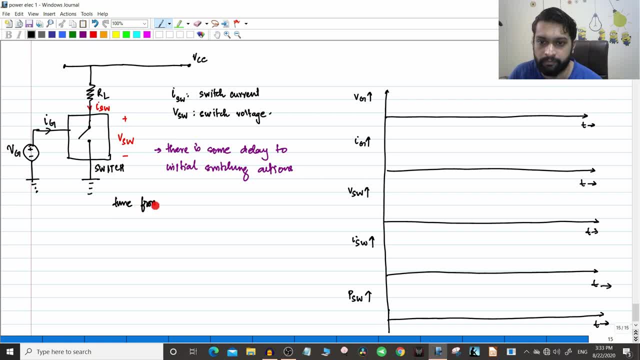 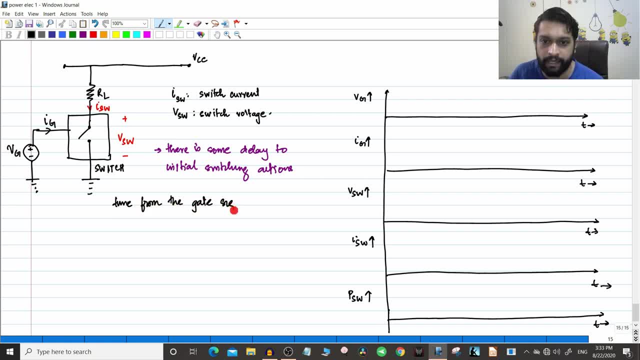 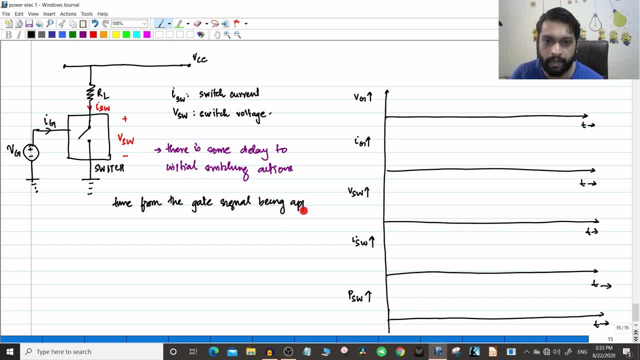 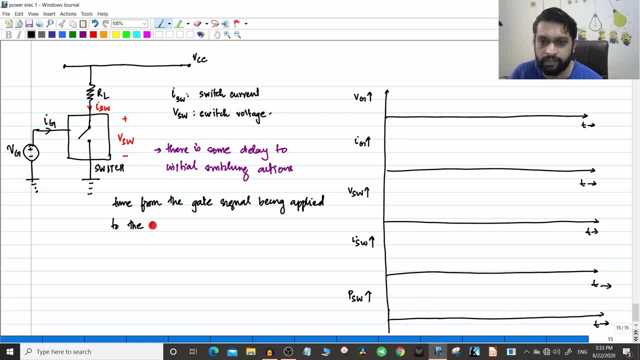 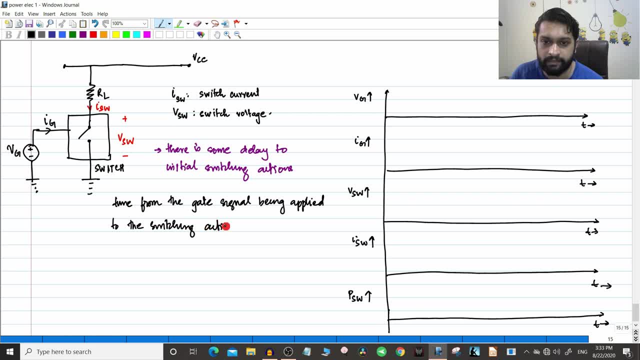 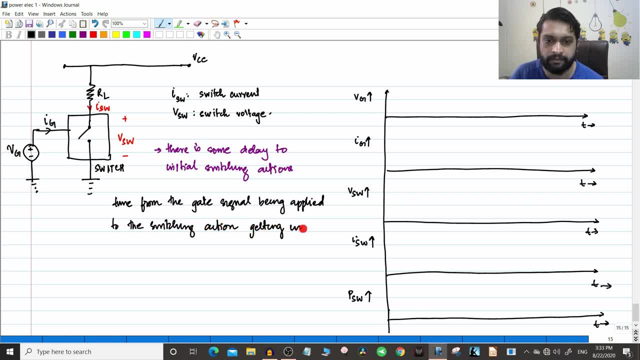 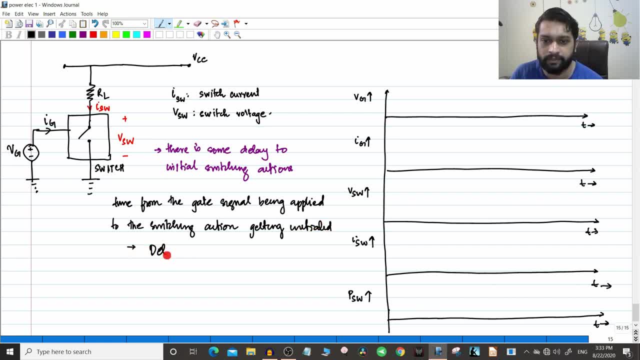 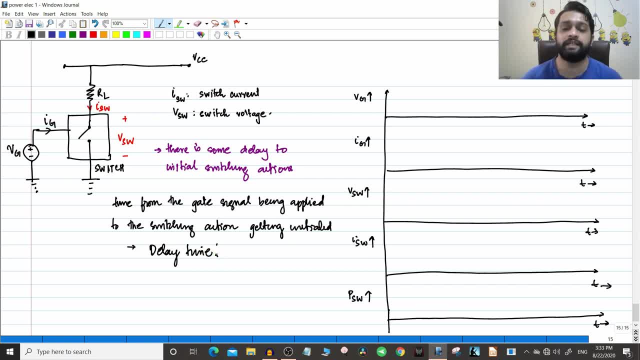 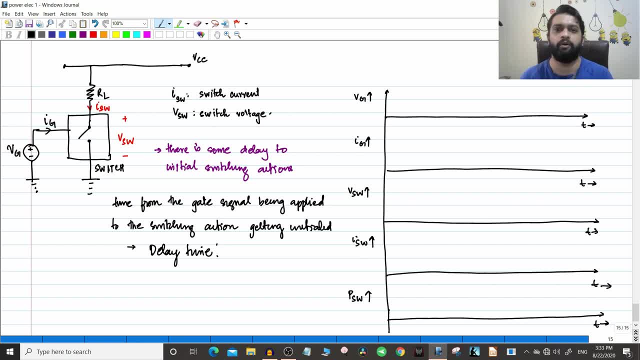 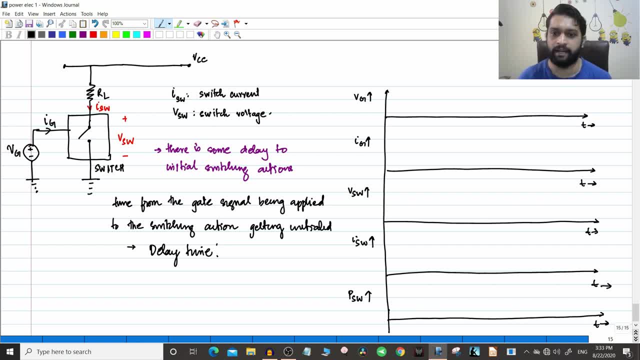 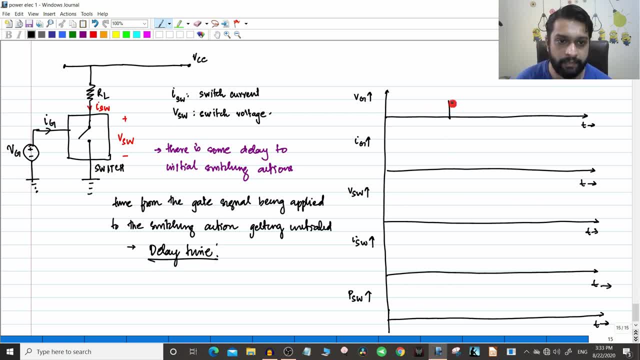 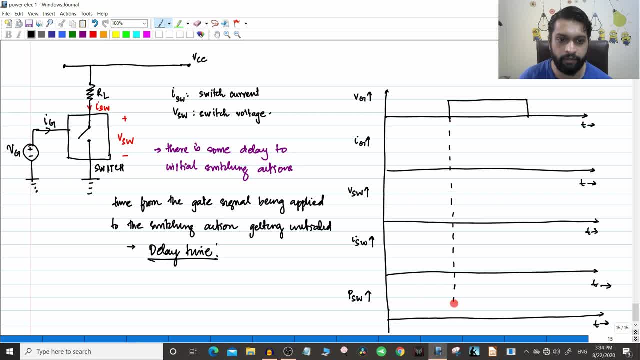 t1.. So in this video we will just introduce a few terms like delay time, rise time, etc. So that we can move to the proper graphs in the next lecture. So this is t1,, this is your t2.. So what is t1?? The gate signal is applied, the time when which the gate signal 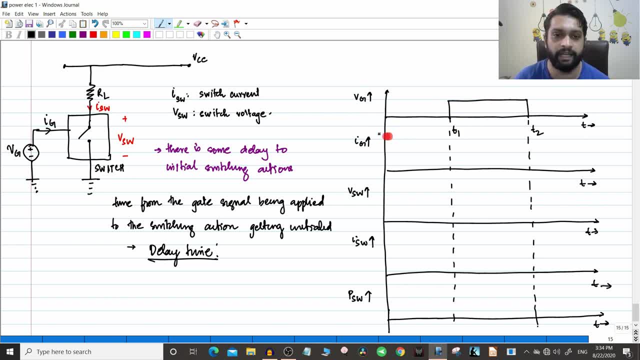 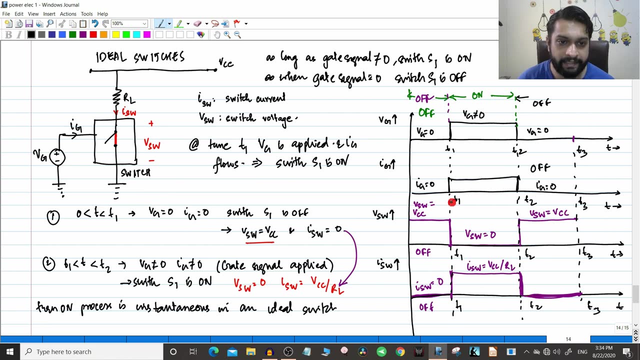 is applied and this is vg. this vg is the gate signal and ig is the gate current. So here, this is the gate current, So the on action will be from t1 to t2.. Now, what I have told you in the previous graph, you see in the previous graph, you see exactly. 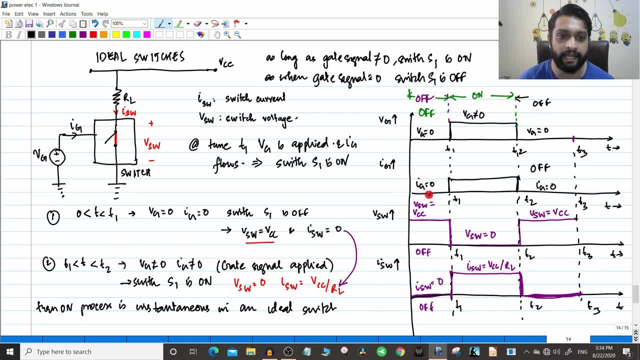 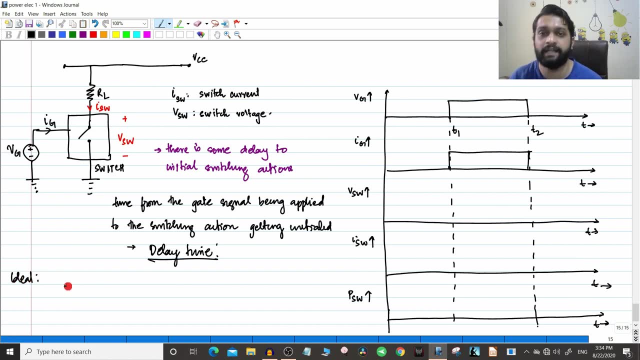 at t1, vsw came from vcc to 0,, exactly at t1, it came from vcc to 0 and exactly at t1, it came from. isw came from 0 to 0. So we will just write down that in the preview, in ideal characteristics, in ideal characteristics. 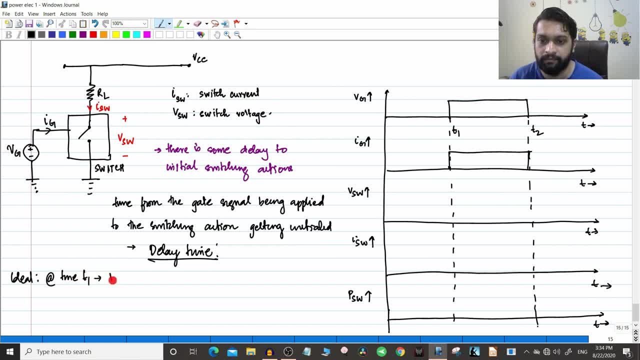 at time t1,. at time t1, vsw moved from vcc to 0 and isw moved from 0 to vcc divided by r. Now what we are telling it will not do it at time t1, it will do after a small time. 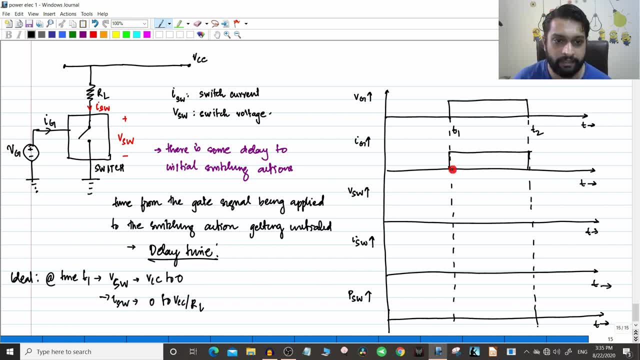 interval. Okay, So let us assume that after this point here, actually what should the graph have been? I will draw that in a dotted line. Okay, Actually the graph should have been like this: So at off period, off period- vsw was equal to vcc. So it was equal to vcc At t1, it becomes: 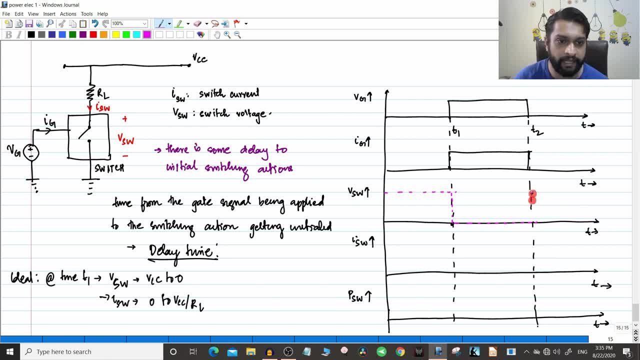 0, vsw becomes 0.. So this was the ideal graph. and here again the graph, and let us not take the next trigger. Okay, Let it be like this. Okay, So this is the turn off, turn off to turn on condition, And what does app happen to? 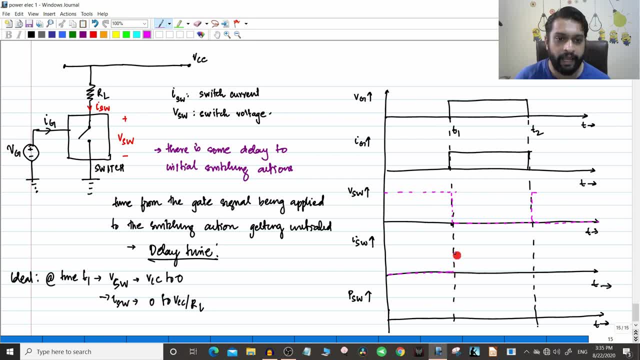 isw. isw current was 0 during turn off condition and at turn on condition it was increasing like this and it became vcc divided by r. okay, Yeah, anyway, yeah, we can show that it to be equal to. I have anyway close the gate. 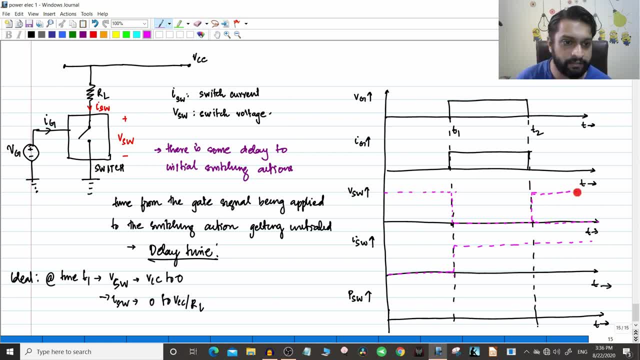 signal here, right, So here also it is turning for. so we can dry it like this. Okay, sorry for that. So here also you can just rub it. So after t2, it is turning off, right. After t2, it moved away from the unit edge signal toimt to r-t1, there is no change. After t2, there is no change. After t2, it moves. 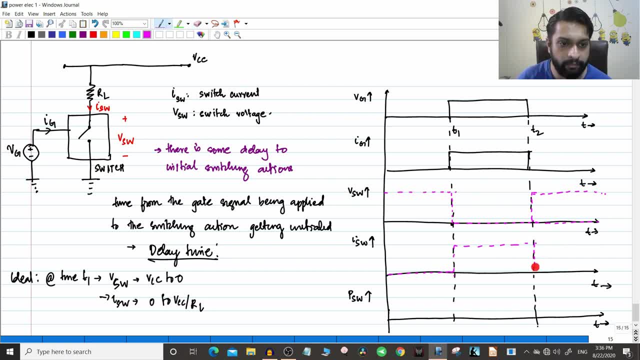 So after it is t2, it is turning off, So the current will become equal to 0. So I can show it like this: So that is okay, So this was our ideal case, what I am telling. 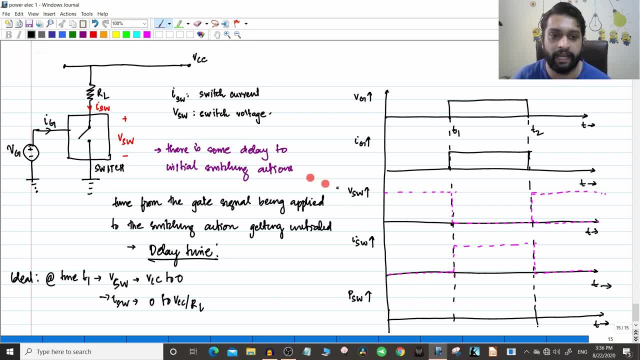 is that it will not turn, that switching action is not going to start at t1, it is going to happen after a delay time. Let us call it as delay time td. So this is your t1. And let us start. let the initiating action start at this point here. So this time interval. 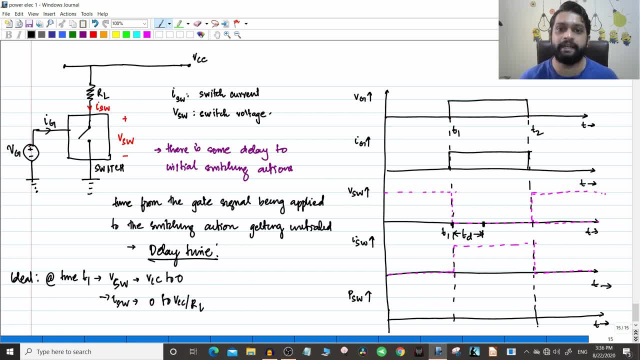 from t1 to that time where actually that happens is called td or delay time. So this is initiating, see this area. this t1 is where switching action starts. After some time, td, the switching is going to actually start in practical case. So the characteristic: what will it look like? 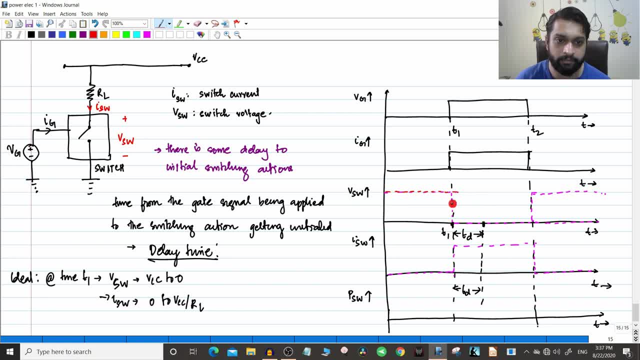 so it will look like this. So it is. it was supposed to come 0 at this point, but now it will come 0 at this point. at td Vsw. It was supposed to come 0 at this point t1,, but now it will delay itself a little bit. 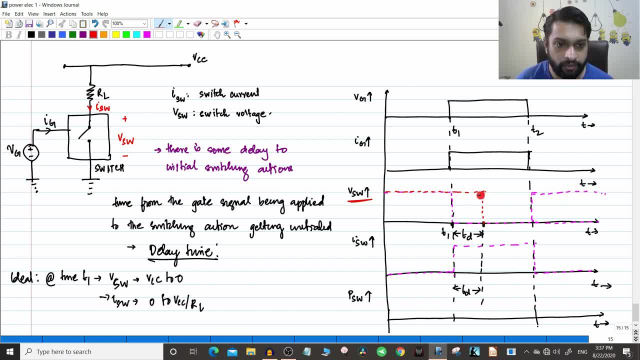 and do it at a time interval: td. So this is the actual characteristic. After delay time it will come to 0,. it will go like this, And let us only take till this point here, Because here we have to define some other terms that we will do when we are going to. 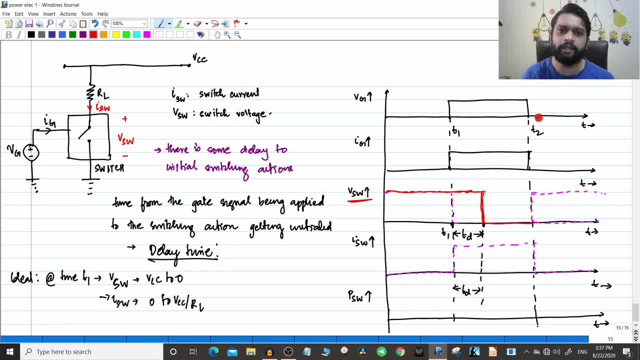 define the actual characteristic. There is a small time. we will define that here itself. So once the switch is turned off. once the switch is turned off, it should instantaneously go up right Vsw should instantaneously go up to Vcc when the turn off is happening. But here also. 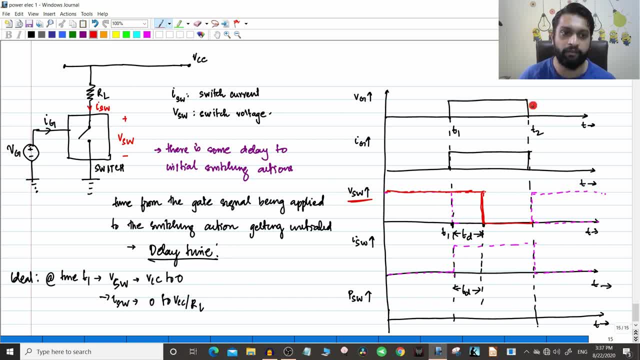 it will not do instantaneously. Once the switch is turned off, that is, after t2, it will take a small amount of time and after that, only it will, it will actually come to Vcc And this time is actually called ts, or it is called the storage time. That means the 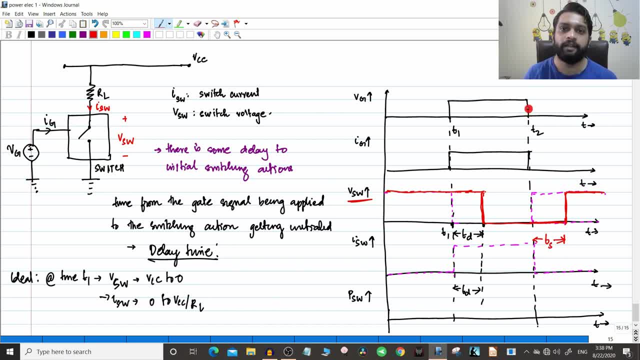 point from which there is time delay. So this is what it will essentially do here For this particular switch. here it should go once the switch is turned off, it should the turn off has happened and the time at which the actual turning off is happening in the actual 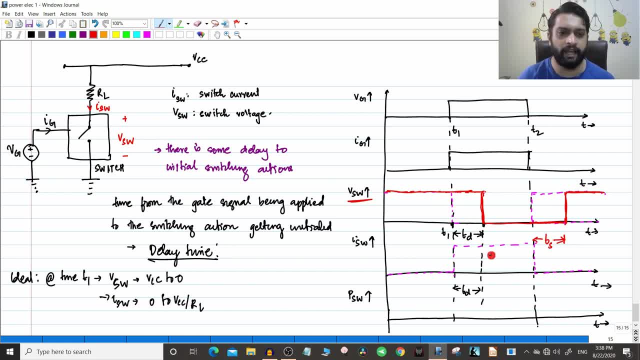 device is called Ts. You will see this properly in another graph. So it is ok, Let us draw it for the current now. So the current: see T1,. the current was supposed to go from 0 to Vcc divided. 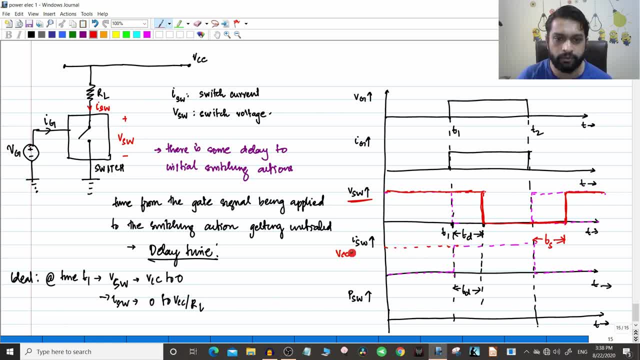 by RL. It was supposed to go to Vcc divided by RL at T1.. But I am telling that it will happen after some time. So this is off condition: current: 0, 0, 0, 0, 0.. At this point you are. 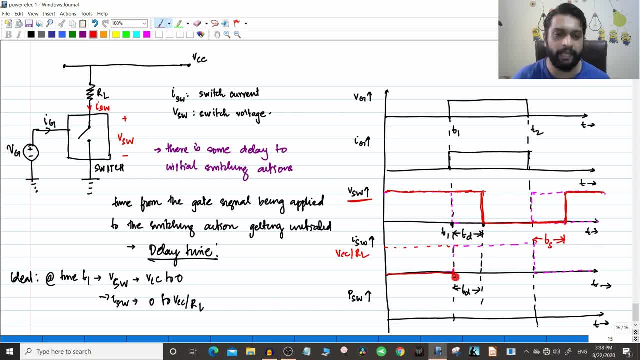 supposed to jump and go to Vcc by RL, But what I am telling? it will take some time, which is called the delay time, which is this point here, And after that it will become like this, And it will continue like this, And at this point, T2, the current, was supposed to be equal to 0.. You. 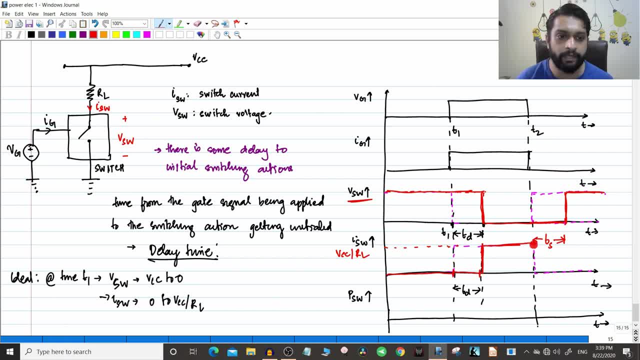 see the previous graph: at T2, current would come to 0.. But it will not become 0.. It will travel a little bit more And at the point Ts it will come to 0, like this. So this is also called the storage time Ts. So we saw the delay. 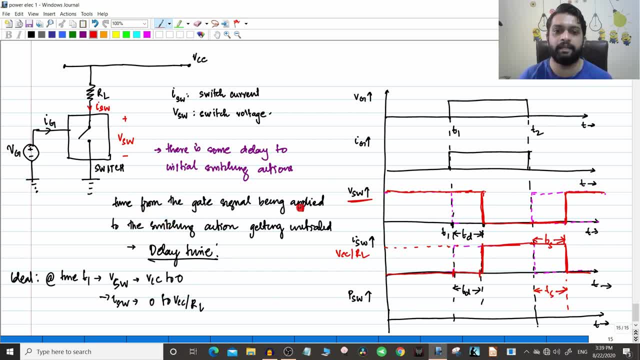 time and the storage time. So delay time is the time from the gate signal being applied to the switching action actually getting initiated, And what is storage time? The switching has turned off, The switch has turned off, But or the gate signal has been removed But for the actual action. 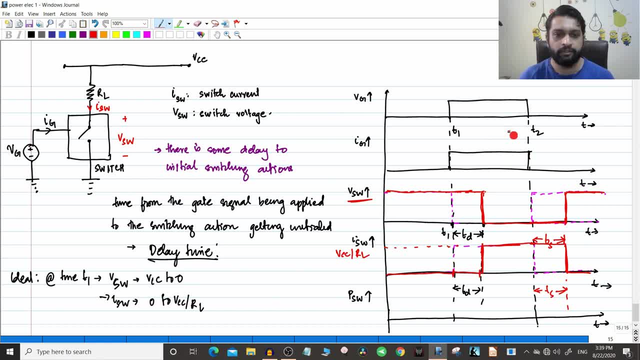 to happen, how much time it is going to take. That is called the storage time. So this is introducing one element called the delay time. So this is the delay time. So this is the delay time Here also one thing we have assumed, That is, once the switching action is taking. 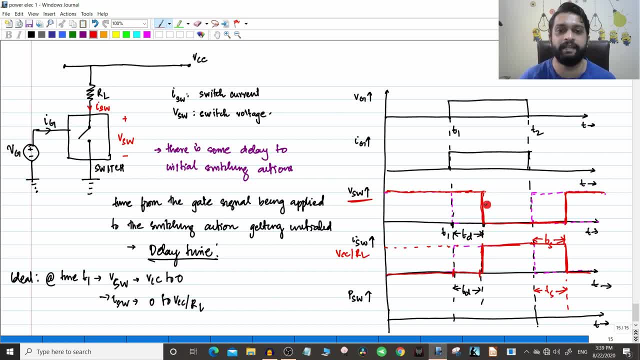 place at Td. once the switching action is taking place at Td, it is instantaneous. There is no delay in the VSW becoming from this point VCC to 0. This is instantaneous. This is instantaneous here. So now we have to assume that that switching action, that is, the VSW, value going. 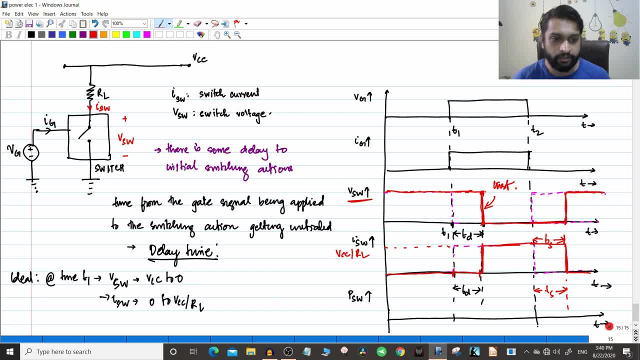 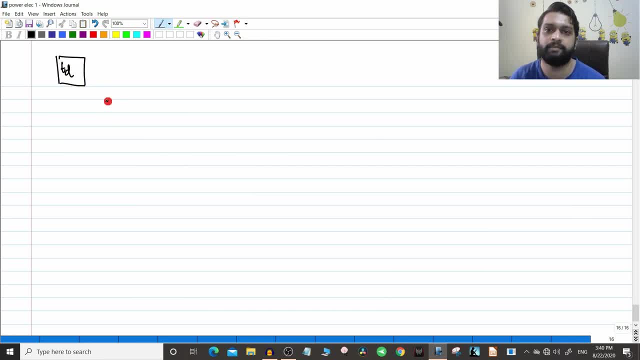 to 0 also will take a finite amount of time. So what we have done here is that we have assumed there is a delay time Td. We have assumed that the delay time Td is there, But after the Td, after Td, the action is instantaneous. The actions are instantaneous. VSW goes from VCC. 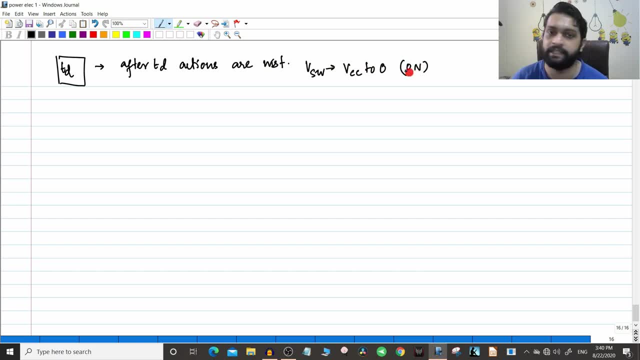 to 0.. That is the turn on condition instantaneously. And ISW goes from VCC to 0. So, So that is the delay time. So after the Td the action is instantaneous. So even after going from 0 to VCC divided by RL, that is the turn on condition instantaneously. 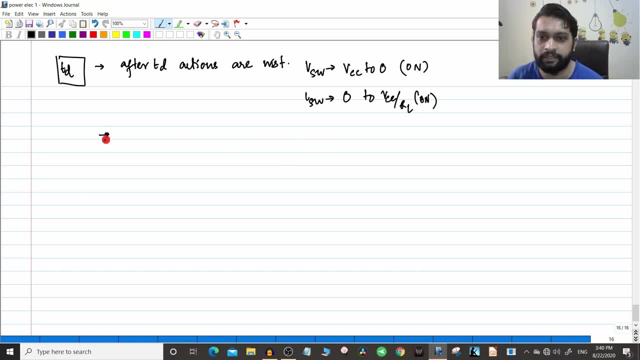 Also in the OFF condition. we assume that after a time interval of Ts this is the turn on condition make for the OFF condition. we saw after Ts the actions are instantaneous. The actions are instantaneous, That is, VSW went from 0 to Vcc. that is the off time. and ISW went from 0 to Vcc. that is the turn off time. So in this case the cycle is: mogę is prohibitive so that Vcc goes inherit the SE in all times of Td. that stays the same hours per change over T. solutions are improbable for values If the Z changes after ATT times and between 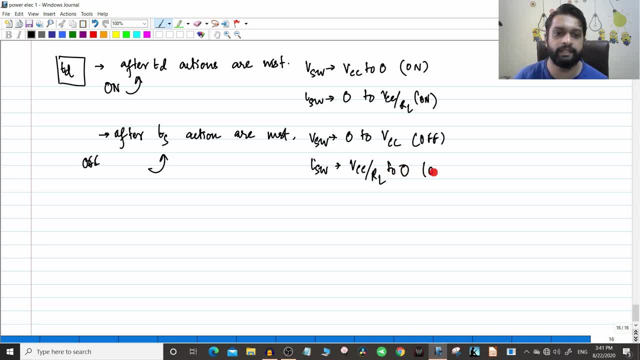 action and outstanding values. the sequence fee varies If, unfortunately, transparent levels are prison and variables went from VCC to RL to 0 instantaneously, that is, in the off time. So this, once that time was reached, action was instantiated, But in real practical switch after the action. 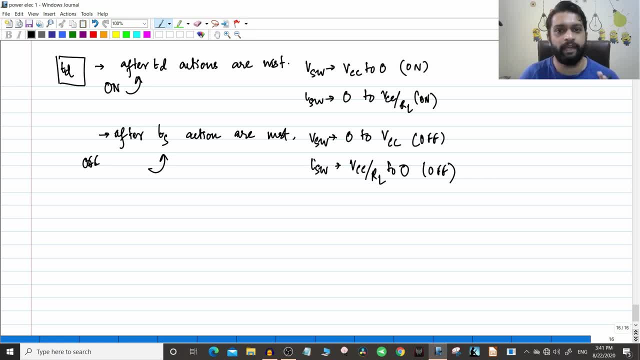 has been initiated. also, it takes a finite amount of time, So that we will do now So that nonlinearity also, we will bring it into the graph, So we will just take the graphs on the previous page and we will come back. So now I have drawn the entire graph, keeping 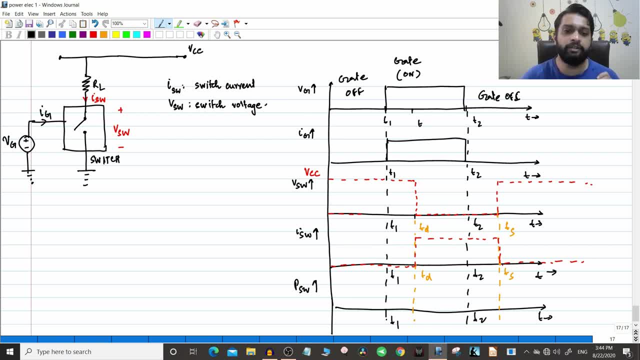 the delay time, nonlinearity. Now we are going to introduce a term which is called the rise time, which is called the rise time In the ideal case. I already told you that the rise time was assumed to be equal to 0. So now the rise time will be the time once. 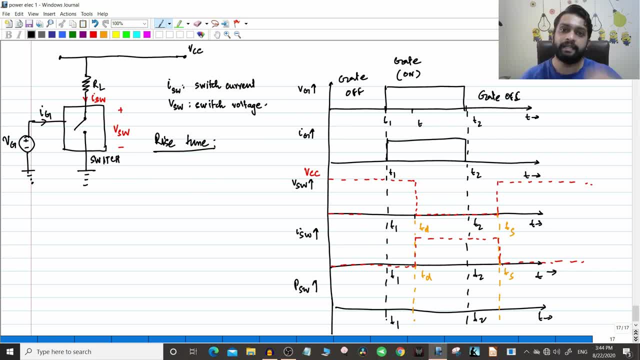 the switching action starts, that is, after the delay time till the switching action completes. So it is the time once the switching action starts, that is, after the delay time time. once the switching action starts, action starts to the switching action getting completed. 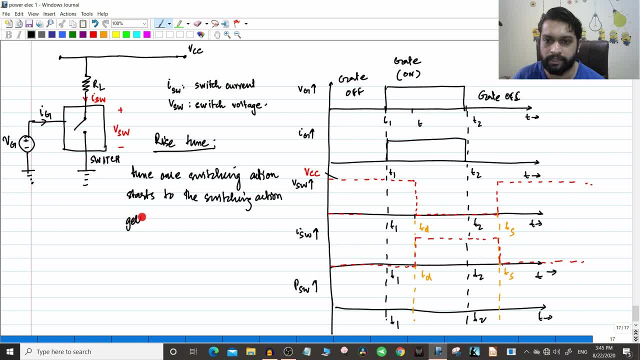 switching action getting completed. In this case it is off to on. usually the rise time is defined from off to on and fall time is defined from on to off. so off to on. So we can also tell it from the switching action taking place to the switch getting turned. 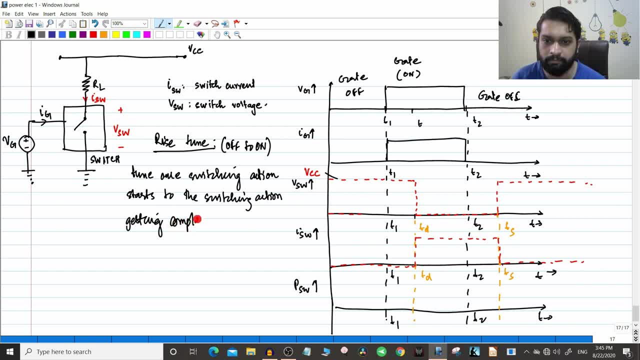 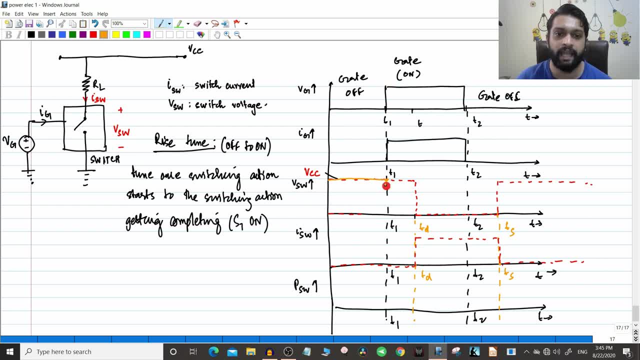 like this: Here you are applying the gate signal at T1. you are applying the gate signal actually in ideal switch. what will happen at this point? VSW will be equal to 0, VSW will be equal to 0. But because of delay time, I told you the switching action will gradually come. it will. 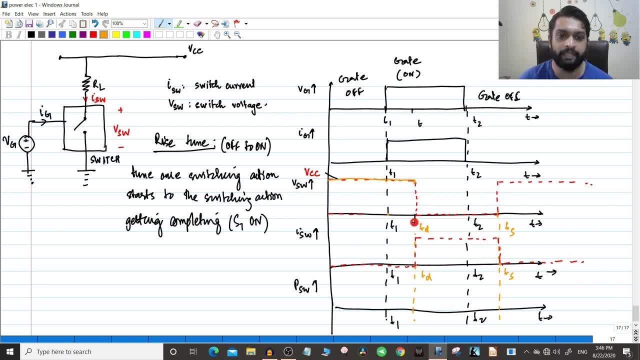 gradually start. At this point again, I told you that it is happening instantaneously, so we have reached delay time. What I am telling? it will not go instantaneously down. VSW will not become 0 instantaneously. it will gradually do that. see, it is gradually doing that, So 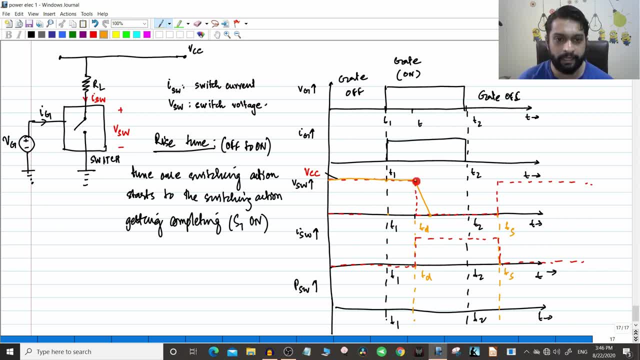 after some interval. in this case, what happened? from TD directly it came to 0,. now it is gradually coming and at this point you call that time interval as TR. So from TD to this point you call that time interval as TR. So at this point the switching action has taken place. 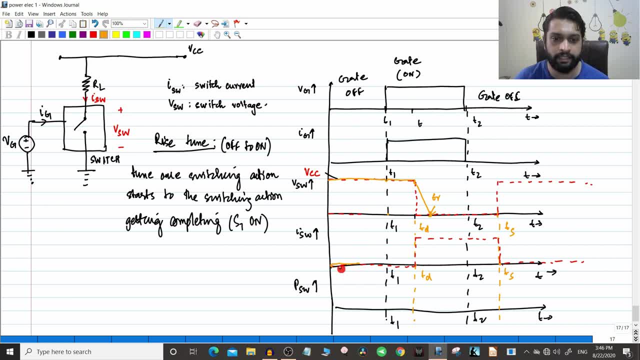 Let us draw it for current. So current is 0. during off condition: 0, 0, 0, 0, 0.. Here, T1, the switching action has to start. gate signal is applied at T1.. So the current was: 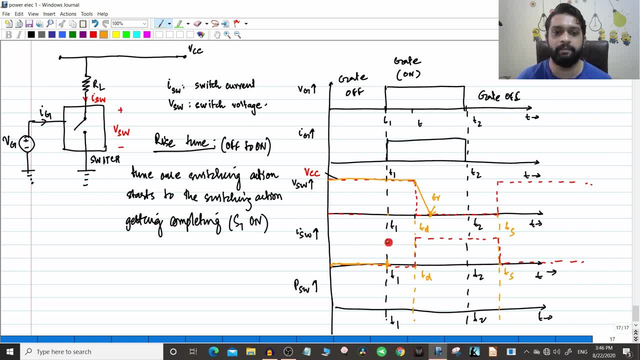 supposed to go like this. it has supposed to increase to VCC divided by RL, But because of delay time it is delayed like this. it will come till the delay time Here. I assume in the previous case it was instantaneous. So in the previous case TD was not equal to. 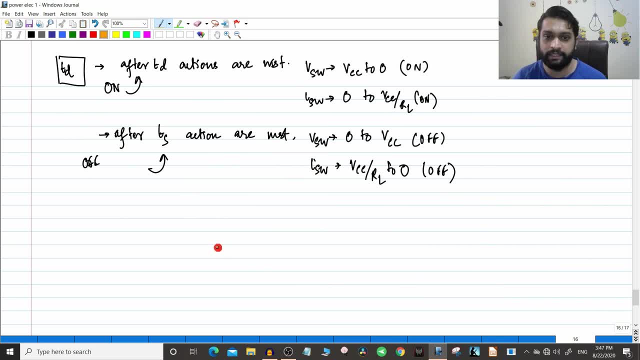 0, TR was equal to 0. So we will write down there. So in this case, what we assumed TD to be not equal to 0, but we assumed TR to be equal to 0. So that was for this graph. 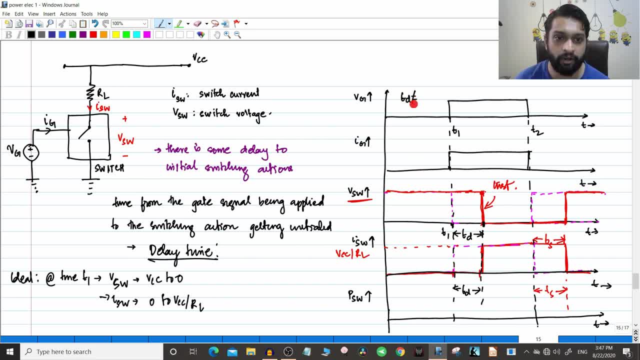 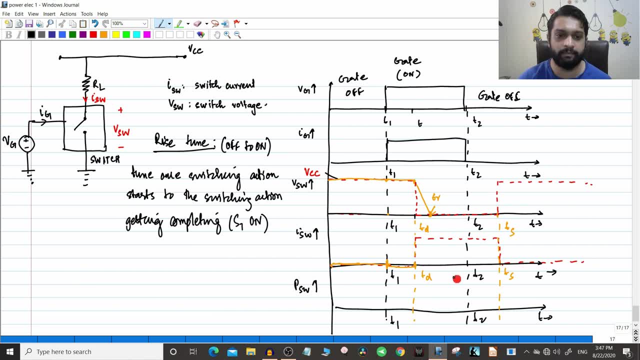 This graph is based on the assumption that TD is not equal to 0, but TR is equal to 0, the rise time is equal to 0. So this is how we are developing the subject's role. At this point. what happens? The current is not instantaneously rising, it is gradually. 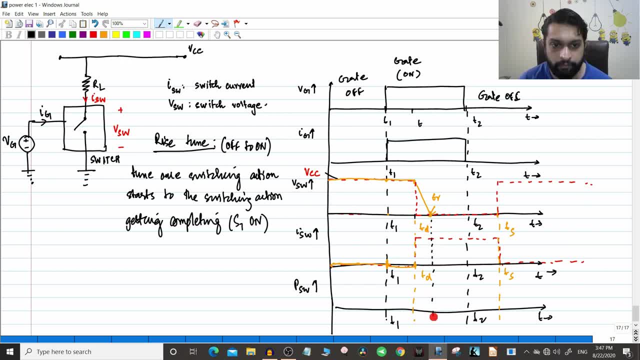 going to rise And these two, the fall in the voltage and the rise in the voltage, we are taking it as to be the happening in the same time interval. So here the current will gradually rise and it will reach Vcc divided by RL, at time tr, So this is Vcc. 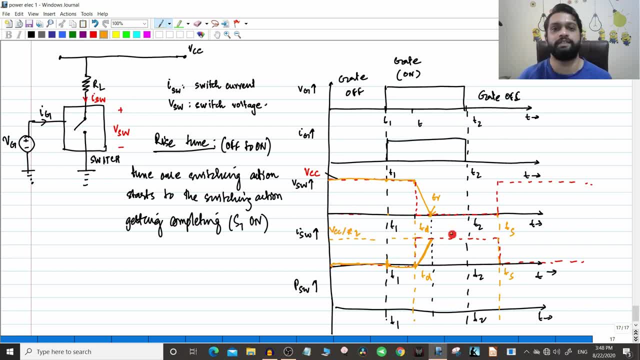 divided by R. So the switching action is completed. The switching action is over now. So now, once the switching action is over, what will happen Here? the switch has completely turned on. At this point now, after tr, the switch has completely turned on, So the actual 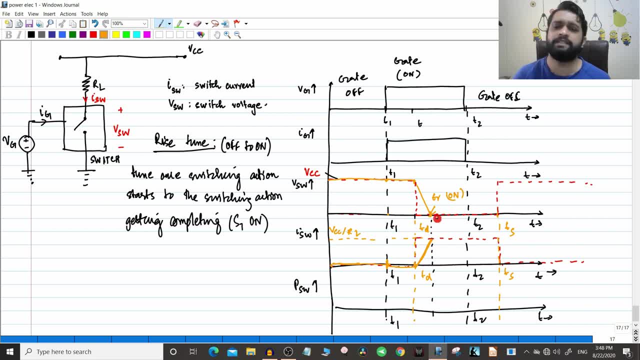 turning on has been completed. at this point, TR. Once it is turned on, what will happen? VCC will be equal to 0 till this point. At this point, what happens? Gate pulse becomes 0.. Gate pulse becomes 0.. What you are expecting. 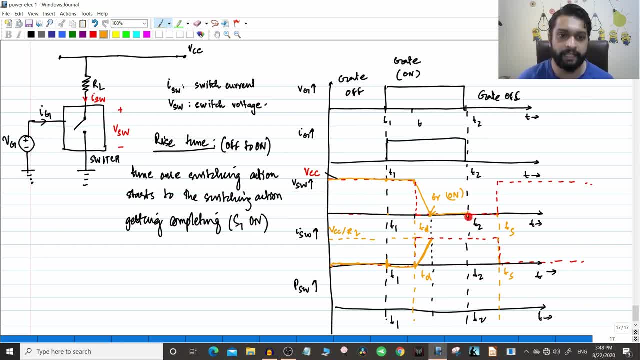 It should go to VCC After T2, after the gate pulse has become 0, you are expecting VSW will become equal to VCC. We have already seen that, But it will not happen. Why? Because of storage time. So it is gradually going to come like this till storage time After. 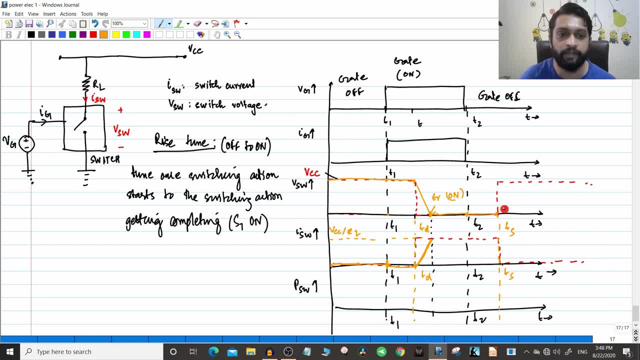 storage time. we assumed that the previous experiment, what did we do? Instantaneously it went up. No, it will not happen like that. It will gradually happen And that time period is called the fault time. So here, from off to on, we have seen. Now again from on to 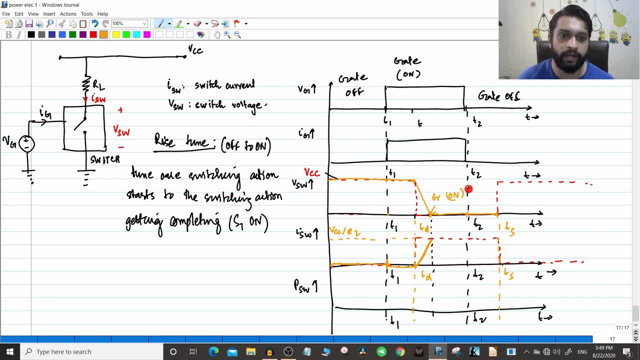 off. now switch was supposed to go from on to off condition at T2. But it did not happen because of storage time, And at TS also it is not going from on to off condition because of something which is called the fault time. So here it is gradually going to rise. 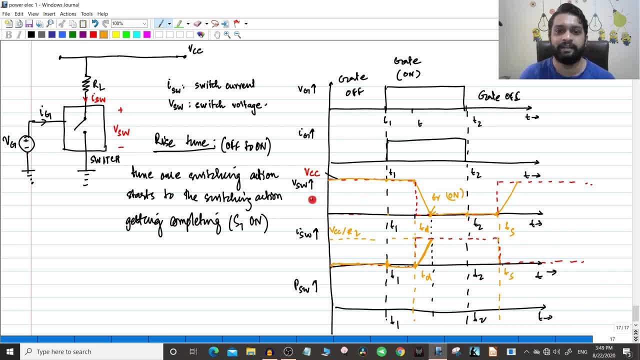 See rise in the sense. do not think that the switch is getting turned on. Whenever switch gets turned off, VSW will become equal to VCC. So that is the basic idea. So here, after a time period of TF only, the switch is completely turned off. 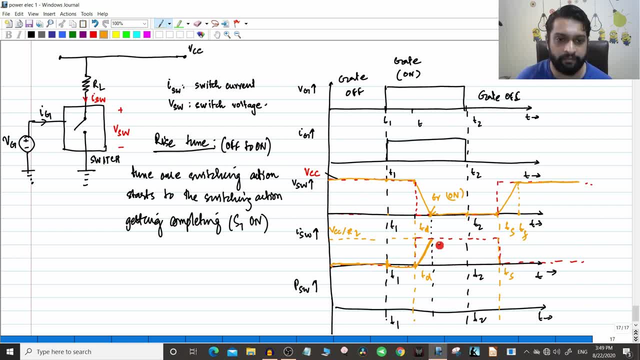 It is like the graph is like that. Let us see for the current graph. So now the switch is turned on, So the current is VCC divided by RL. At this point the switch was supposed to turn off, but it will not happen because of storage time. that on condition is maintained. 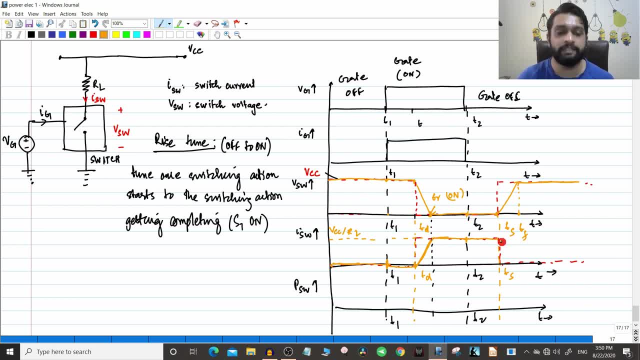 for some more time, like still this point, After this time, after the storage time also. it is not instantaneously going to fall, It is gradually going to fall. That is, the current is gradually going to decrease from VCC divided by RL to zero, Just like the voltage gradually. 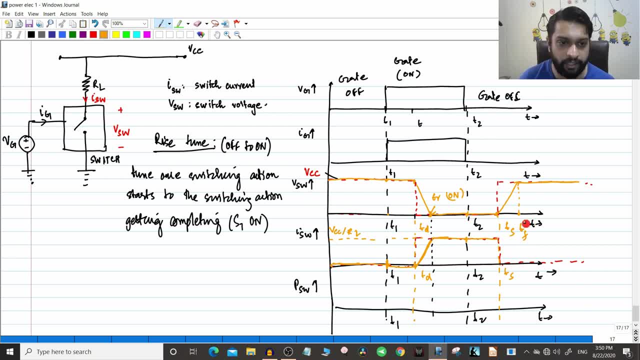 increased from zero to VCC. The current is gradually going to fall down and it finally, at TF it will become equal to zero, like this. Beyond that we are not seeing the graph. So to explain it once again, we will start with the current waveform. So from zero to 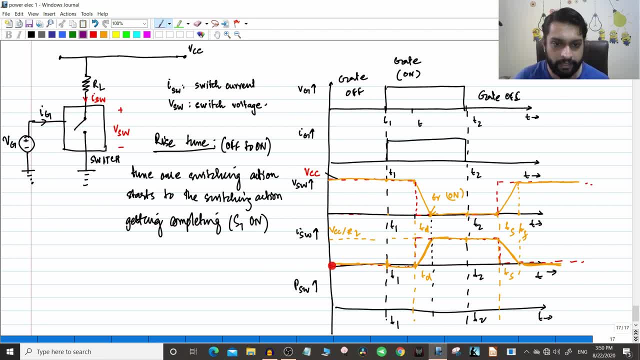 T1, the gate is in the off condition, So we will take a red color pen. So from zero to T1, gate signal is not there. So from zero to T1, gate signal is not there. So from zero to T1, gate signal is not there. 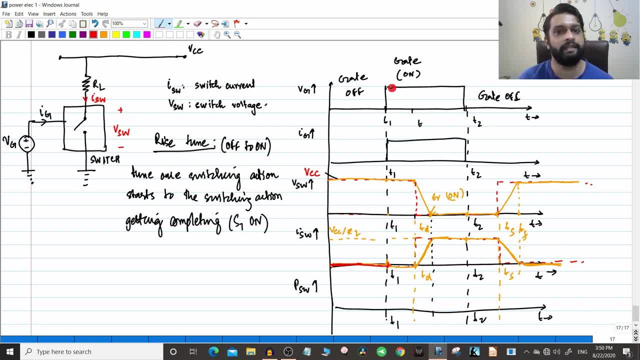 So to explain it once again, we will take a red color pen. So from zero to T1, gate signal is not there, So from zero to T1, gate signal is not there, So from zero to T1, gate signal. 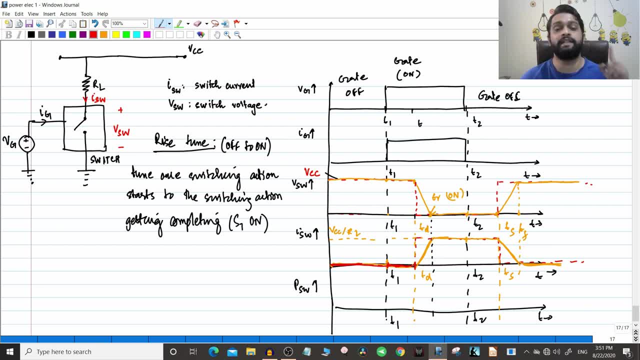 is not there. Here you just apply the인. we mean the let x. it is indeed 0.. So when this attack has occurred, RL goes through. So at T1 the RL goes through, and that is saving time of RL from 0 to T1.. Now how the RL was saved, where, How the RL is got saved and 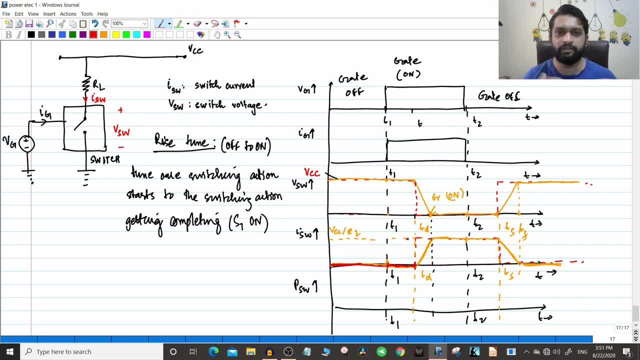 the RL part também gets saved. Finally, let's design a RL onboard, Like vice versa. Of course it will be very, very small, but we can measure it. So once the switch starts to turn on, the current will not instantaneously increase. 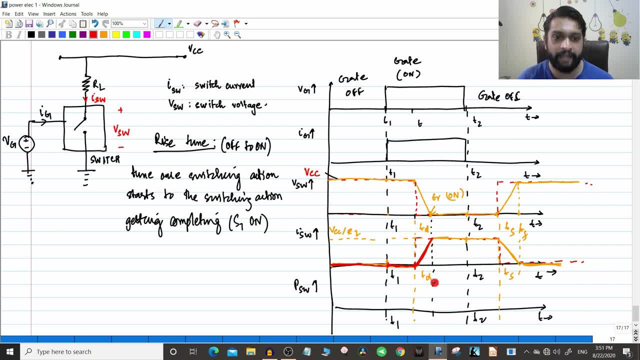 Gradually it will increase to VCC divided by RL And that will complete in a time which is called rise time, From TD to TR. it will take, Once the switch is turned on. current will be how much VCC divided by RL, like this: 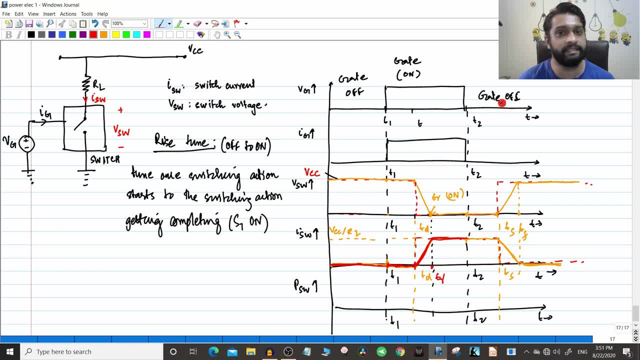 At T2, what happens? The gate signal is removed. At T2, what happens? The gate signal is removed, You are expecting the current will go 0. Because once the gate signal is removed, the switch is turned off, right. 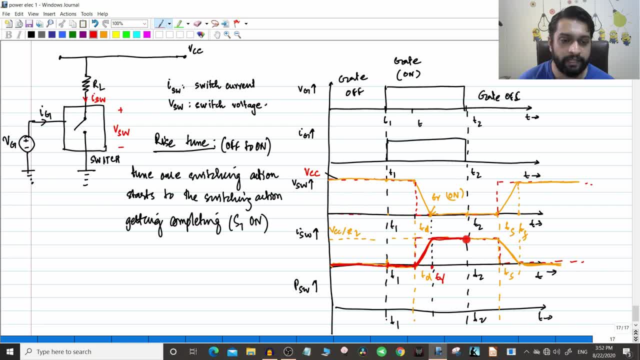 You are expecting current will be 0.. No, it will not happen. It will gradually happen at TS. right, It will take till start Now at TS. will it go to 0?? No, TS, it will not go to 0.. 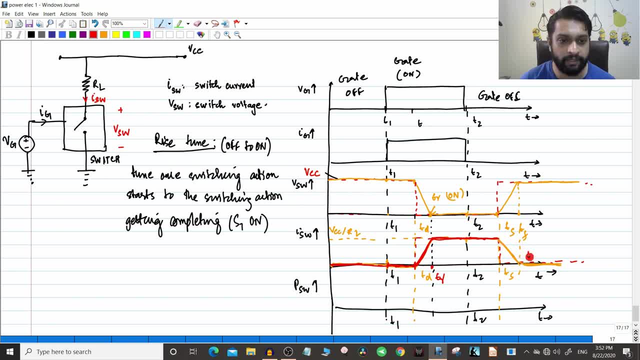 It will gradually go to 0 here, From TS to TF. it will take. So, from TS after a time TF it will become 0, like this: Okay, It will become 0.. And here the Actual turn off is happening. 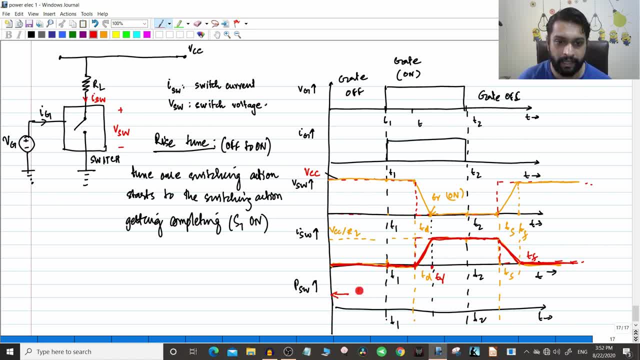 Okay, So actually the turn on of the switch is happening here, So this is the time taken from the gate signal applied to the switch actually getting turned on is here, So this is also called as T on. We will see it in the next graph in more detail. 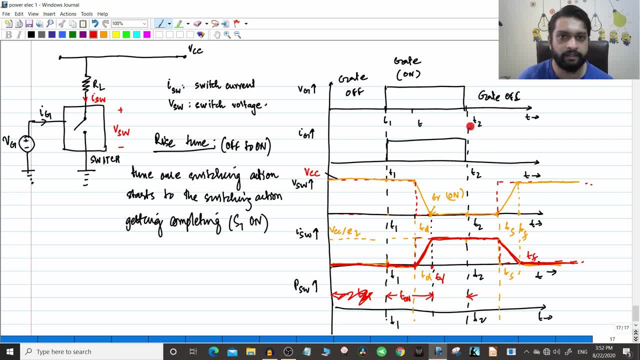 And here at T2, you are turning off. right At T2, you are bringing off the signal, But it is not turning off. So from here gate signal being applied. So from here gate signal being applied. 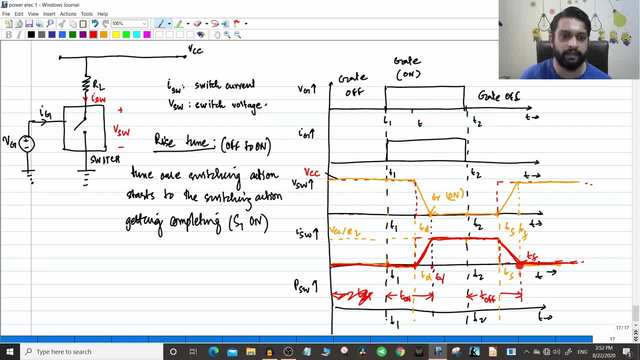 But it is not turning off To actually the switch turning off. that is this point here, TF, it is actually called turn off. So we will see that in much more detail when we actually see the graph. Now we will see it for the voltage. 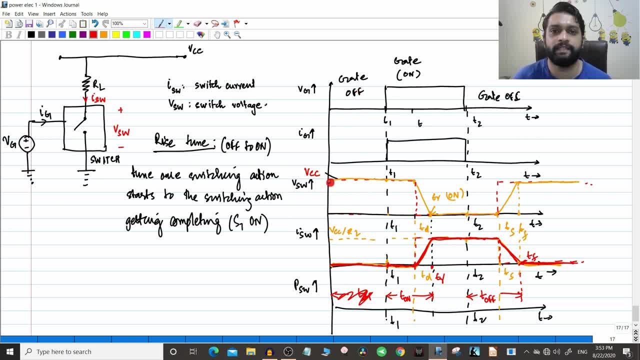 So when gate is off, switch is off. So what will be the VSW equal to? It will be equal to VCC. So VCC, VCC, VCC. At this point T1, the gate signal is applied. 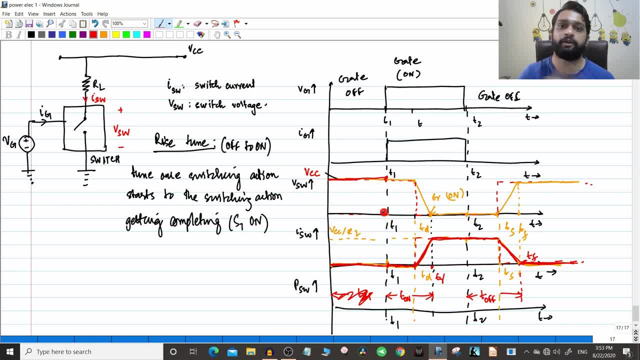 So you expect the voltage to become equal to 0. But it will not become equal to 0. Because of what? Delay time. So gradually it will come to the delay At delay time. will it become equal to 0?? 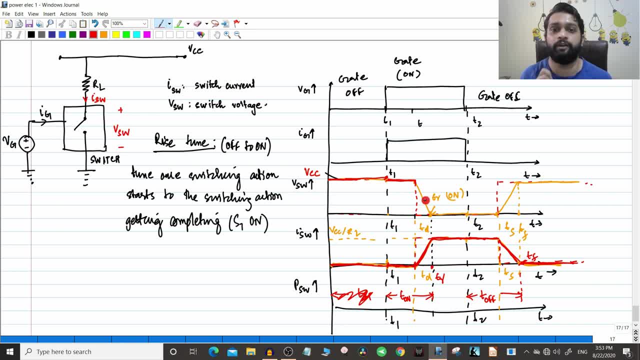 No, It will gradually happen because of the phenomenon of rise step. So, gradually, the voltage is decreasing from VCC And after the time interval of TR, from TD, after the time TR, it will become equal to 0.. So it is going to continue, continue, continue like this till T2.. 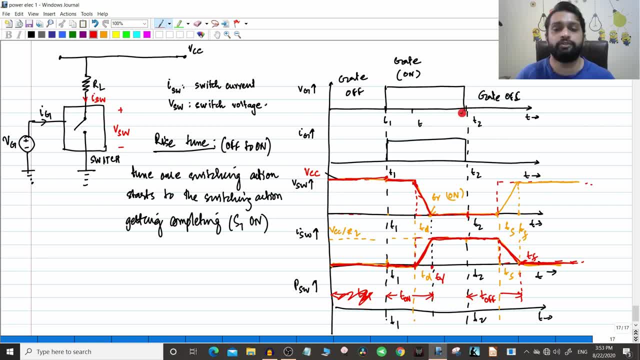 T2, what you are doing. Gate signal is 0.. T2, gate signal is 0. So you are expecting the switch will turn off, But it will not turn off. Why? Because of the storage time. So it will gradually come like this till the storage time. 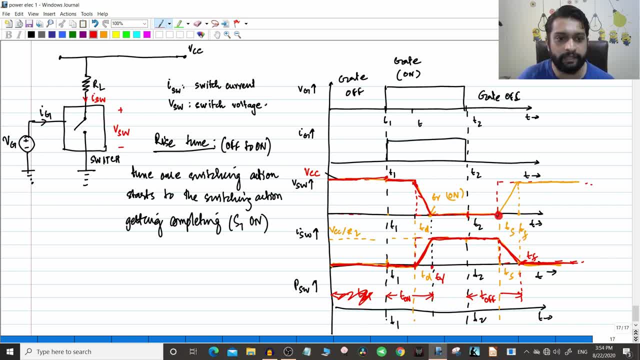 At storage time. the action will initiate Here. also, you will expect suddenly the voltage will VSW will become equal to VCC. No, It will not happen because of something which is called the fault type. So you see, this is the current is dropping, voltage is increasing. 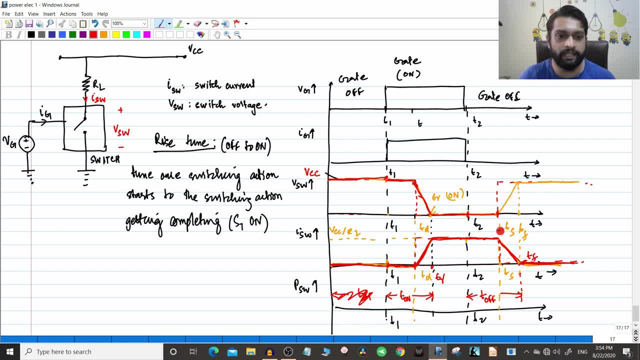 When the switch is going from the on condition to the off condition, current will fall and the voltage across the switch will increase. That will also Take a finite time, which is called the fault time, which is marked by TF, And then, finally, after this point, the switch is actually turned off. 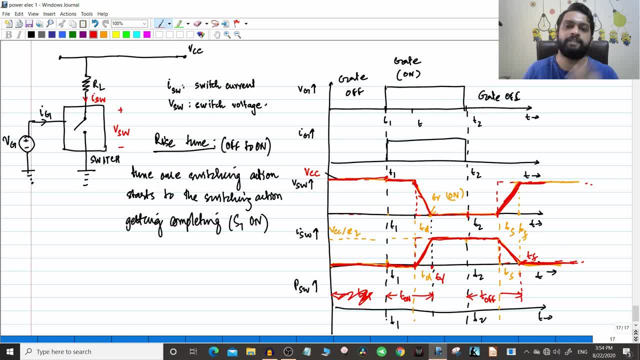 So the instant at which the gate signal is applied to actually getting turned on it is taking a finite amount of time. Similarly, the instant at which the gate signal is turned off and actually the switch turning off takes some amount of time. So this is introducing the terms which is called the delay time and the rise time. 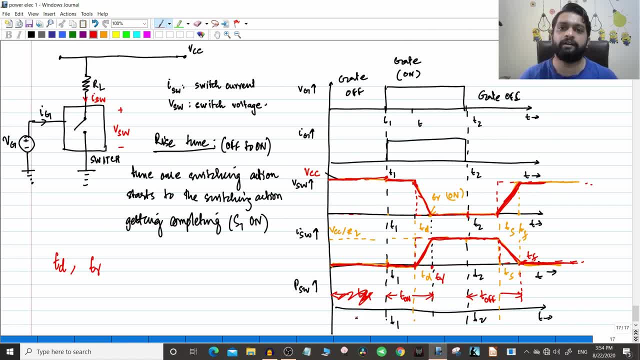 The next video, We will take this graph only and we will draw the graph for the power also- power across the switch- and we will consolidate this into a nice framework in which you can understand the subject more easily. So I hope you have understood this video. 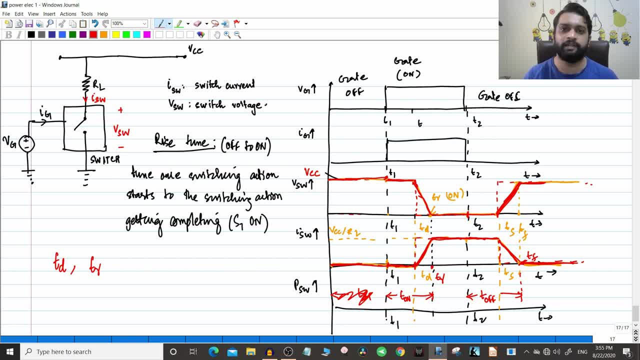 If you have not understood, just go through the video once or twice again, So I'm sure that you will get the idea after that. So till I see you in the next video, it's me, Varun, signing off, and have a great day. 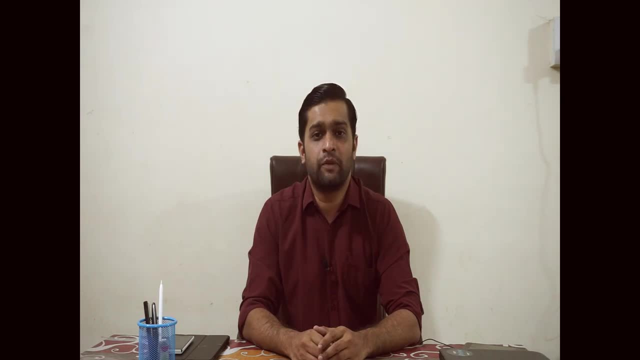 Thank you. Now that the video is over, please stay with me for 30 more seconds Now. the vision of this channel is to create a repository Of good quality videos with crystal clear explanation regarding various topics related to electrical engineering. Now, if you want to help me spread the word, please share this video with anyone interested in these topics. 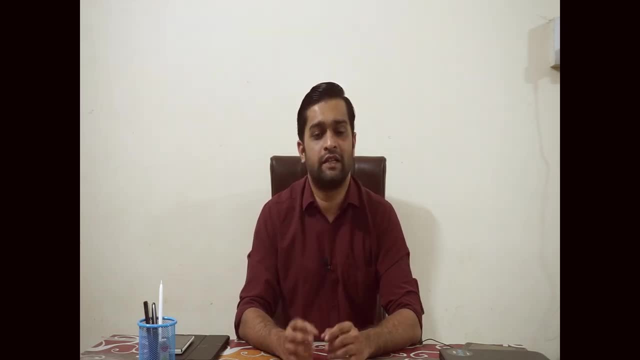 The second thing is that, for me, education is a two way process. Therefore, if you have any doubts or suggestions regarding any of the videos or regarding the channel, please put them in the comments below. We can have a healthy discussion and that way we can build a strong community.